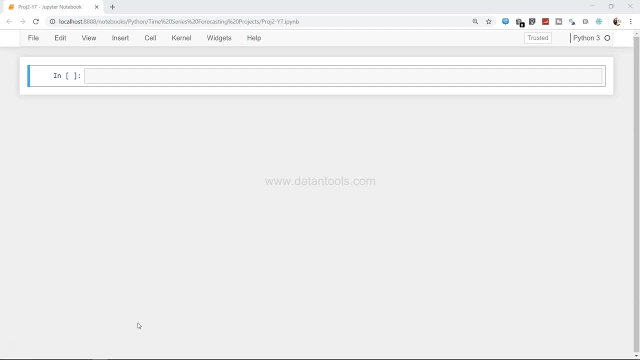 this video right from start to end, and within this we will even discuss some of the interview question that may come when you are applying or when you are giving an interview, as well as during the business scenarios. many times situation comes when you need to give some specific answers related. 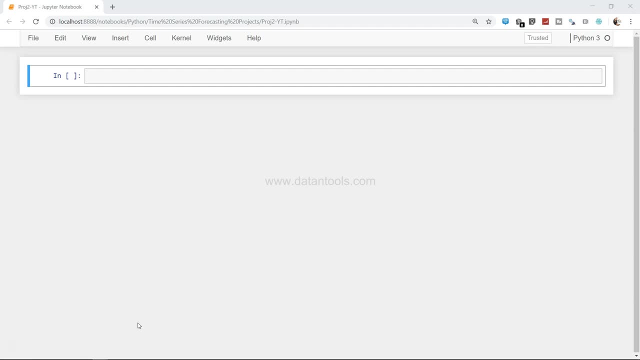 to that and we will see where, as and when the scenario is coming. we will be discussing it. So keep watching this till the end and by the end, give me the recommendation or suggestion in the comments about what you want to see and what. what do you like in this video? what you did? 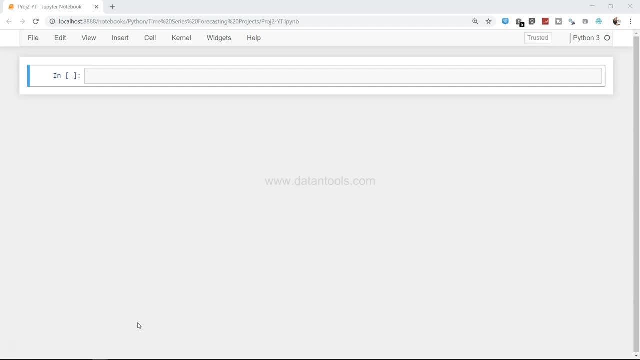 not like and what I can improve upon so that I can give you a better experience going forward. All right, so before. so, without any delay, let's start this by importing the pandas as pd, importing the matplotlibpyplot as plt and percentage matplotlibpyplot and percentage matplotlibpyplot. 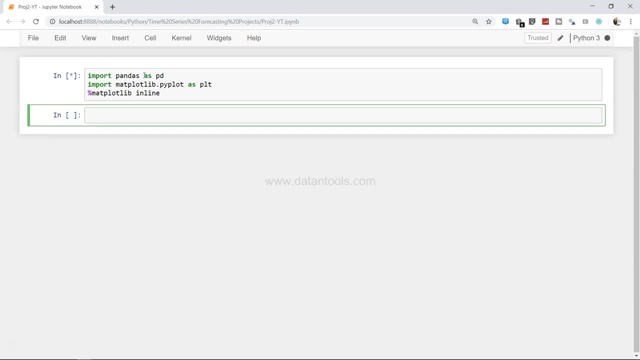 plotlib inline. So these three libraries. one of the very common libraries I am importing- pandas, as you know, for the import of data sets, and matplotlib is to basically plot the data and this percentage. matplotlib inline helps to plot the whatever you know graphics that we want to plot. 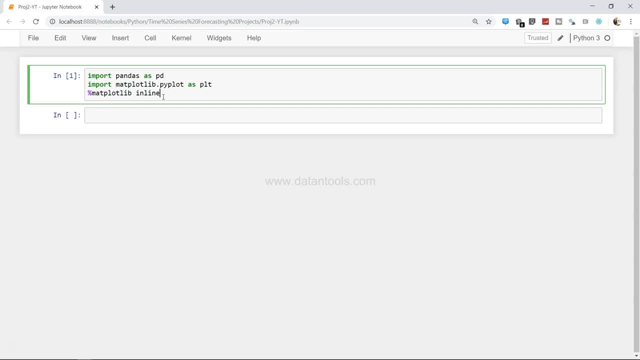 like bar or line chart within the command line built just below to the execution window. Otherwise, if we don't have this, we will have to use, like a pyplotshow, which is a separate command altogether, and I just want to avoid writing more and more code. but we just want. 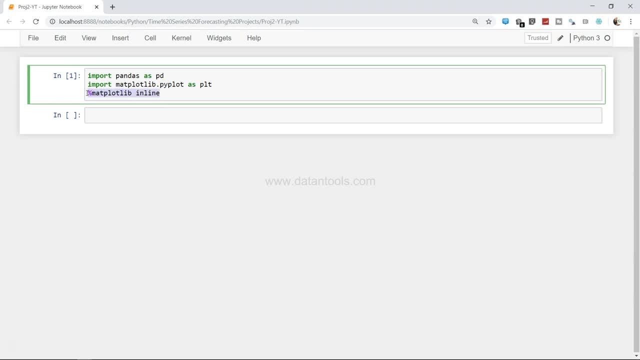 to optimize this entire process with the help of percentage matplotlib inline. So now, with this explanation, if this question is coming into an interview, you know it, why you do it. All right, so let's go ahead and start this. so what do I have is basically a very small 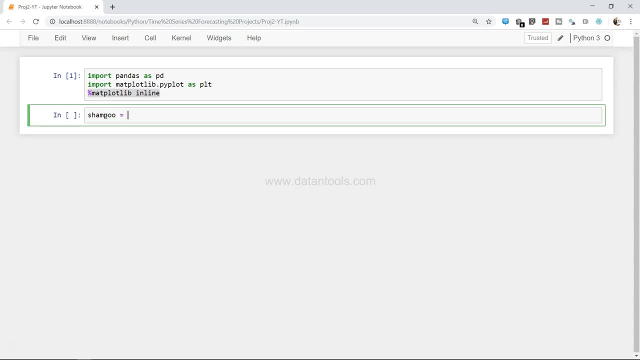 because it is mostly from a learning perspective. if you are here, I'm sure that you want to learn the time series analysis and forecasting, So it's always good to start with a small data set, because with this small data set, you can better understand the data as well. as you know, do much or get a much. 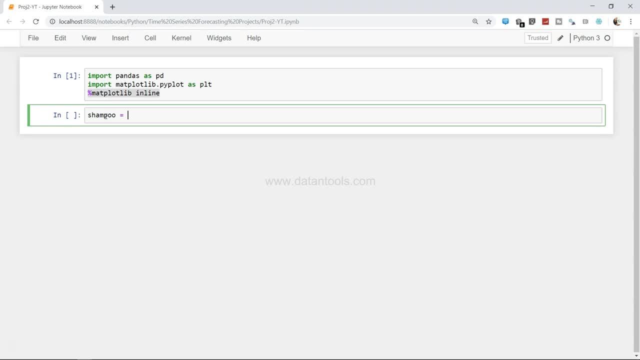 better understanding from all the operations that we will be doing. So, first of all, pdread underscore csv. because it is a csv, So let's go ahead and start this. So let's go ahead and start the csv file. and it is a. it is in the same folder where my this particular file is, So I'll just go. 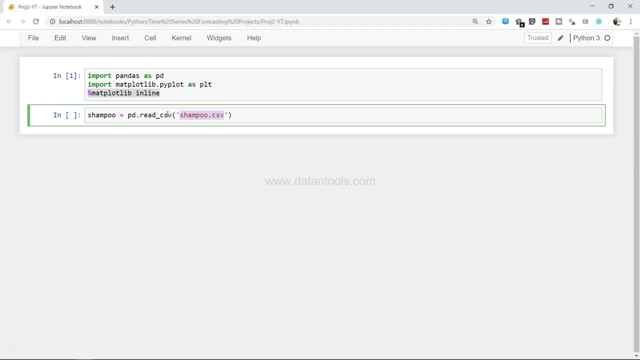 ahead and simply say shampoocsv. if this file is stored somewhere else, like for example c colon- sorry, c colon- forward slash. that should be capital: c users slash- shampoocsv. whatever the path is, make sure you have the forward slash when you provide it, because by default you get the. 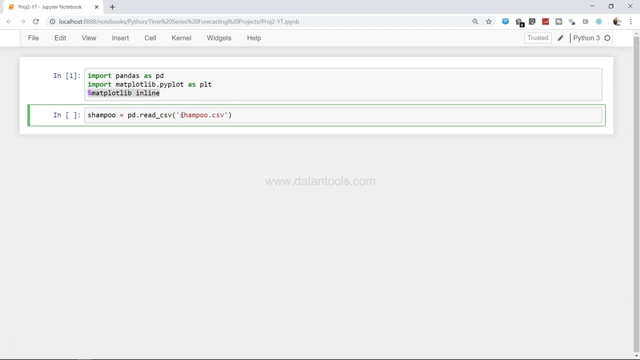 max slash when you are in Windows. so just just to make sure that you have the forward slash. So this is the data set. you can find the instruction to get the data set within the description and for to just to show you what it has is this month and sales, and this is the index number zero one. 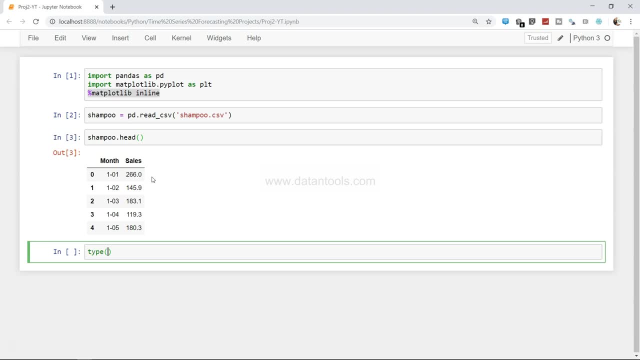 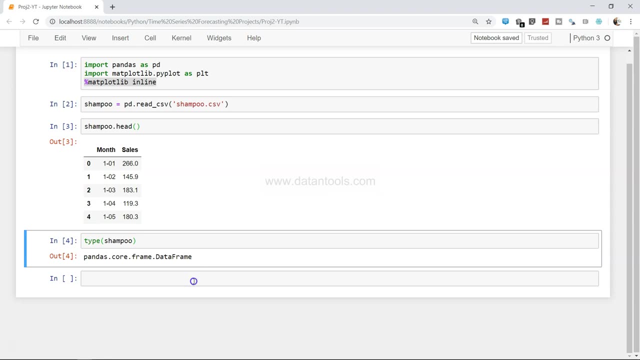 two, three, four. So right now, if you see, the type of shampoo is the data frame, but we need is basically a time series, right? so what we can do is another interview question: how you convert, how you will import the csv file as a time series data set and the parameters. i'm going to 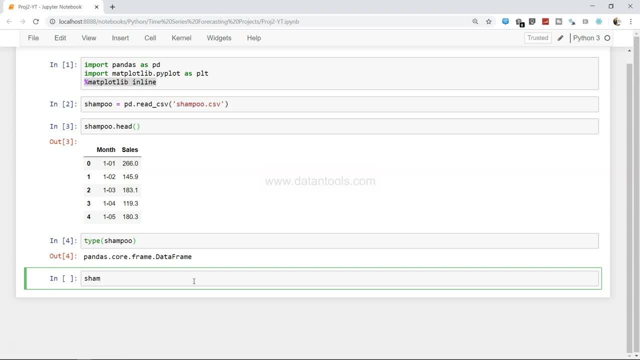 discuss is a very important one, so give a strong focus. i will keep suggesting you, whenever there is something tricky that i'm doing because i'm sure that it may, or it it may come into the interview or for sure they will ask you from a different angle to check your knowledge into the uh, into 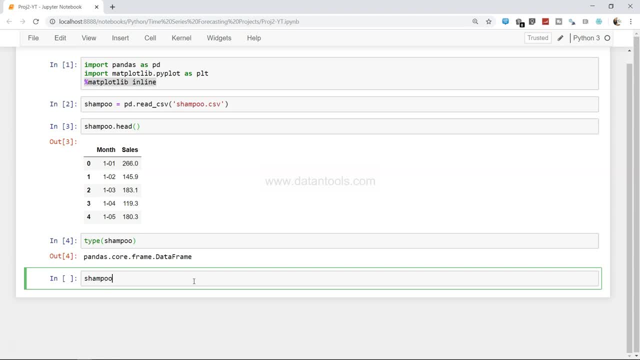 the data import or the data manipulation process. so shampoo and pdread underscore csv: shampoocsv. so what do we need in in this scenario? first is we need to keep the index as month, because our once we do that, we can do a better manipulation of the data. let's say: if you want to search. 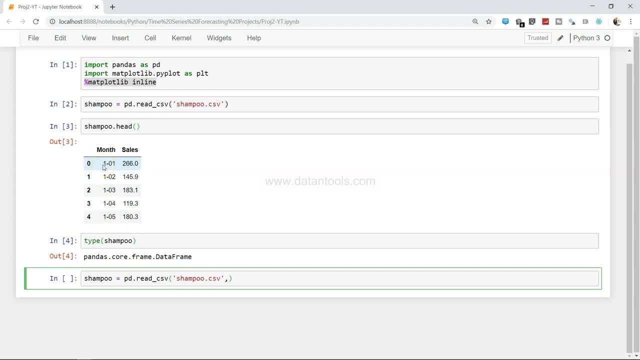 only for the second month. so right now it is first month, one zero one month. two month: one zero two. the second date, third date, fourth date, fifth date. so if you want to see or do a manipulation that a specific point of data frame or a range of data frame we want to see, we can do that manipulation very easily if we have the month. 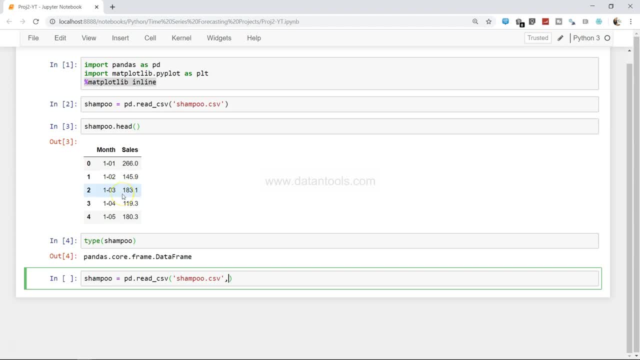 into the index and then we want to make sure that this, this is going into a series instead of data frame. so first of all, we will say index underscore, column zero: this is a zero column and uh, parse underscore dates equals to true. so that means, uh, what we are specifying, that it is a dates column and we want it to be a proper date, and 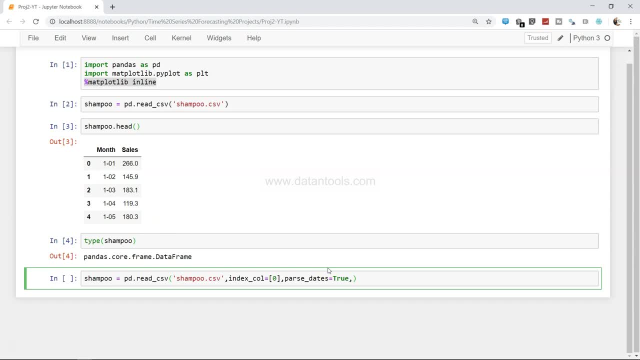 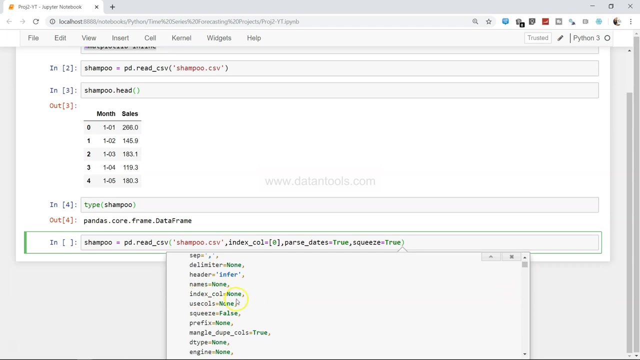 then finally, the important parameter which will convert it into the time series: squeeze equals to true. so if i press shift tab tab, you will see all of these parameters over here. so index underscore, call here: squeeze here. by default it is false, so i have kept captured as true because i want that and parse. 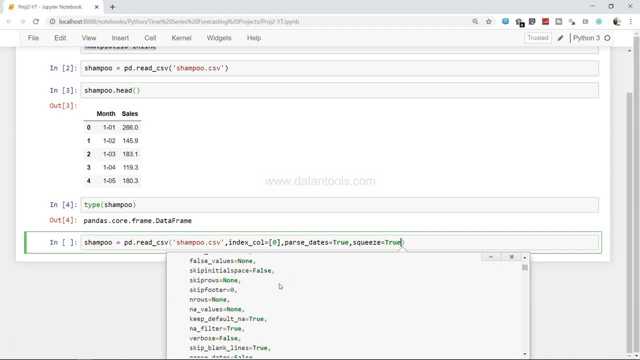 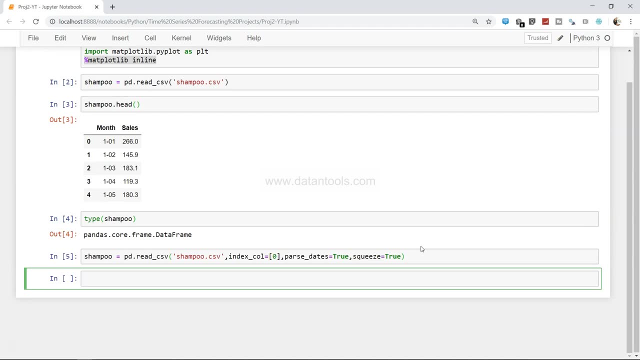 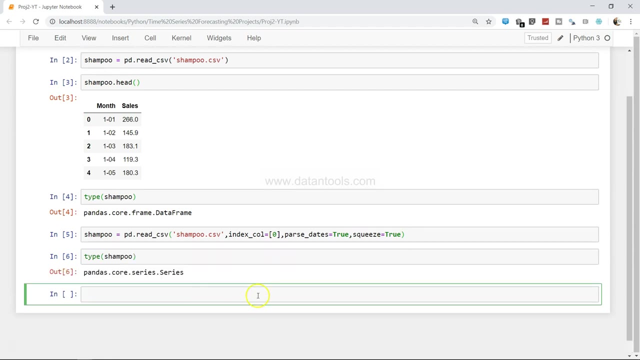 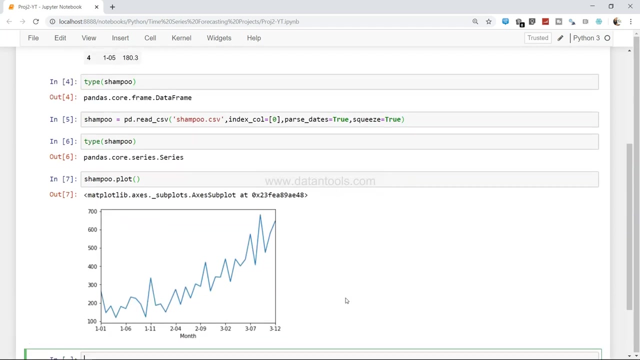 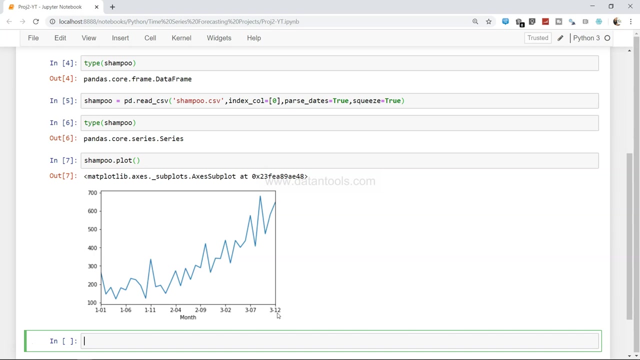 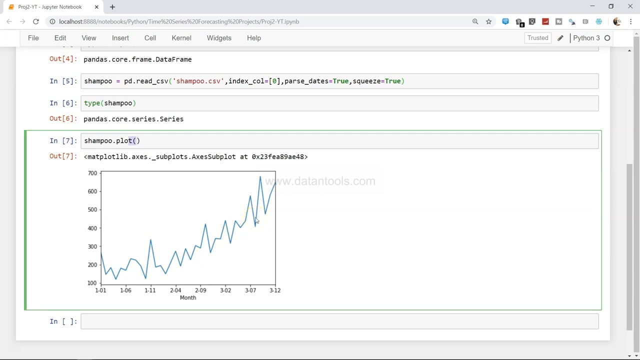 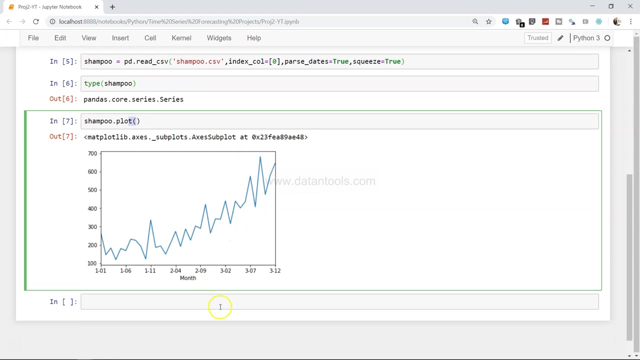 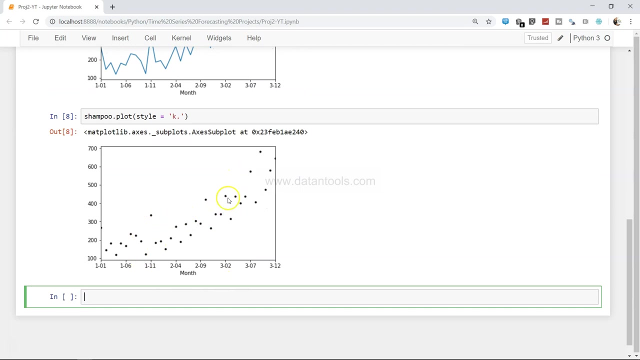 underscore dates should be somewhere. yeah, parse underscore dates is something which i mentioned as true. so if i go ahead and execute it, and now if i see share, share, if i do that, this, this is changed into dots. so sometimes, uh, the dot representation and an easier. 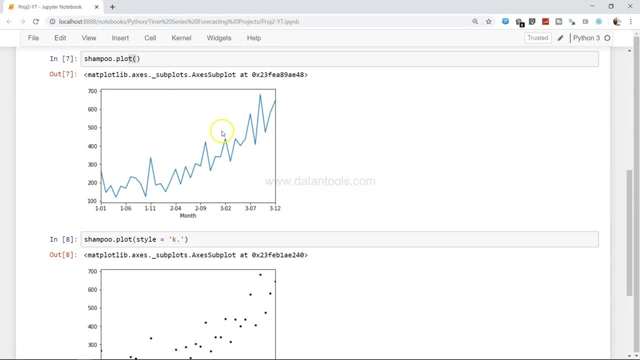 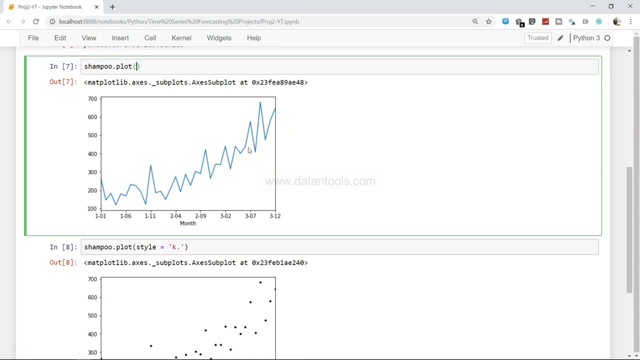 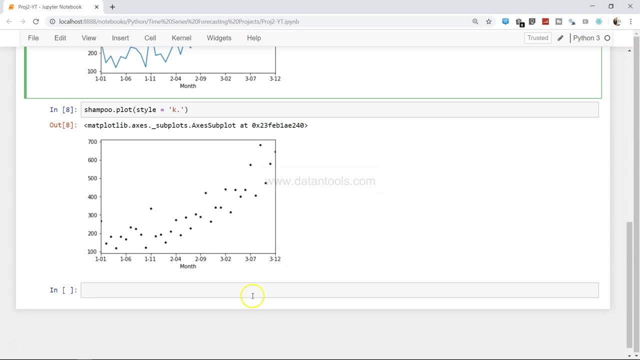 one, and sometimes the line representation is quite easy. default is line. if you see, we don't have specified any parameter. that's why the lining is easy. but sometimes you will see that dot. you know, specifying or having the dots on the plot is something which is making sense. all right. 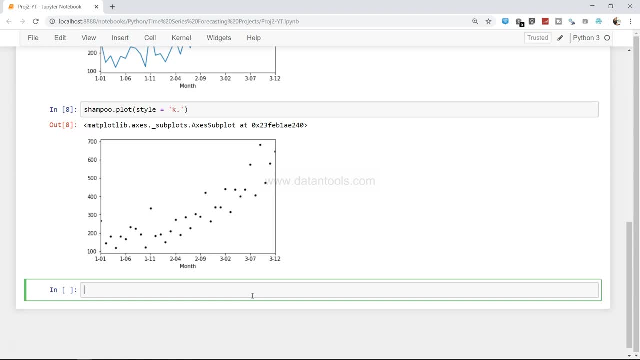 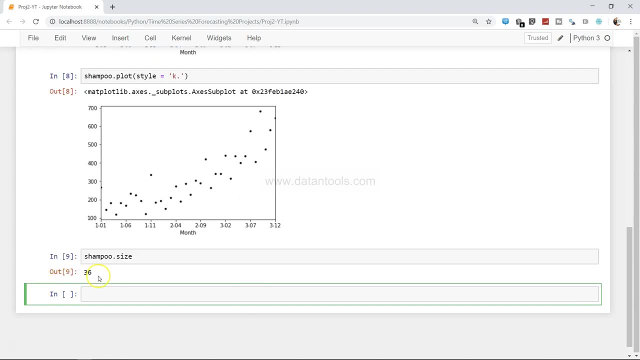 so after that, what we can have is basically just to know how many data points it has. so it has 36 data points- and then, if we want, we can describe it, which will give us a good idea about the statistic of this data set. so this is a see. 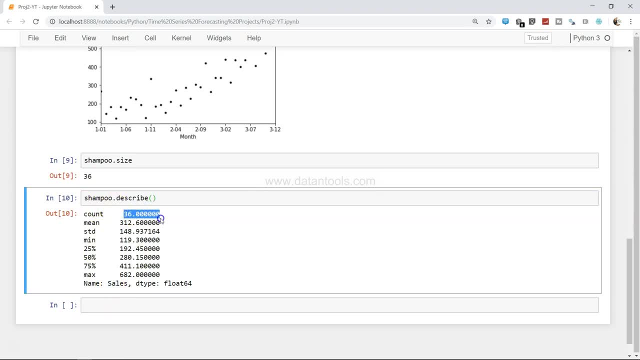 the shampoo data set and total 36 is the count and that's the five data points is and that's what the status is. but we can putload level and equal to letter number and score set was set in FIFA for the totals of data points on the farm again to calculate the data set and total 36 is the count and that's what the игр is the count and that's. 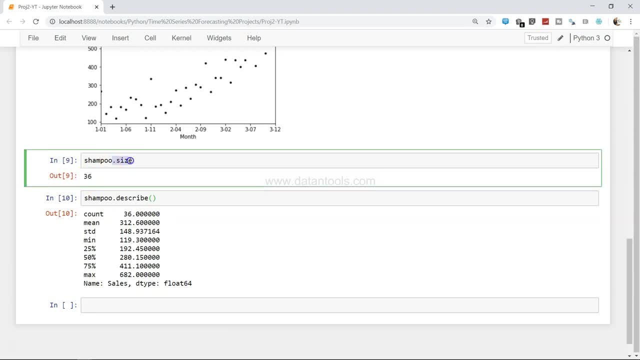 the count over here when we used- sorry, the size method over here and or the size property method. is this- this could be a interview question: what is the difference between a method and the property? so this is a method which has the parenthesis and it can have some arguments as well. 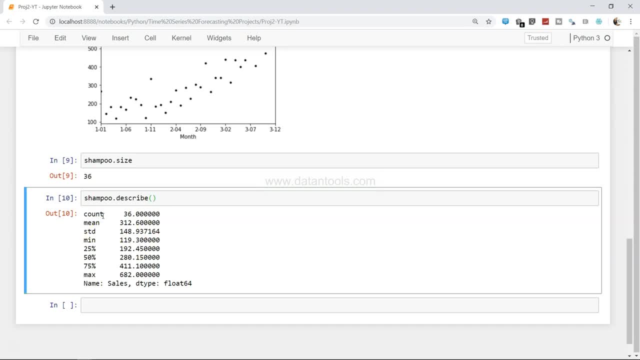 and then we have count, count. is the count simply count? and then the mean is basically an average mean and if you see, 50 percent is basically median, so 280. so what is the difference between a mean and median if? if you don't know this, i highly recommend that you go ahead and just 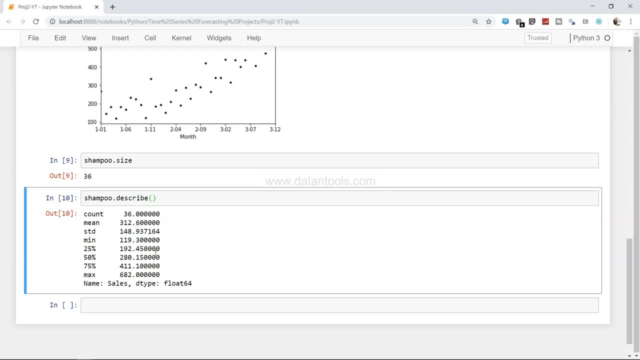 search it because that's a very important interview question. what is the difference between mean and median? and, in a nutshell, if i tell you, mean is simply taking all the values, summing that up and dividing by the count of value, and median is, which is 50 percent median. 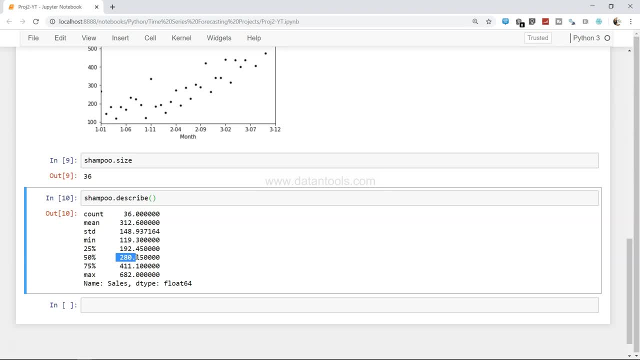 is is simply the fifth, the middle value in an ordered list. so first of all you put everything in an order and then you see what is the middle value. so suppose if you have 30th value, so 15th is your middle, so 15th. whatever the value is at 15th data point, that will be the value over here. but 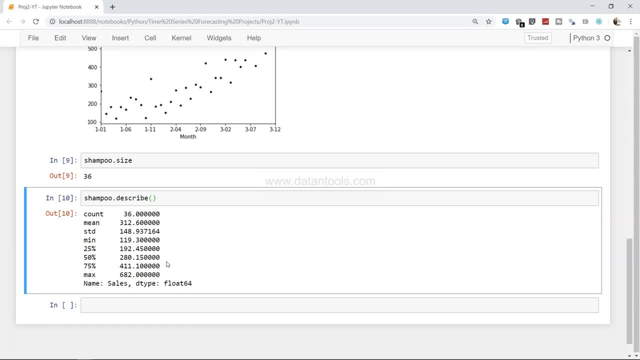 the important is it is an- it should be an- ordered list, and then question arises. the interview may interviewer may ask: okay, if that's the case, then what? what would you do and in which scenario you will use mean and in which scenario you will use the median, and i recommend i can give you an answer. 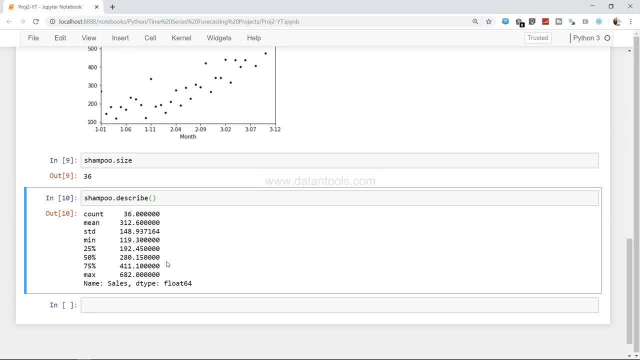 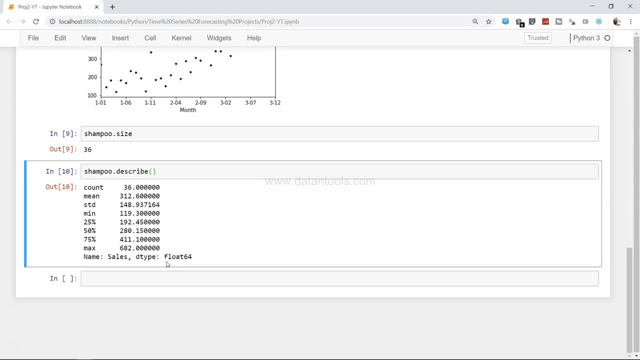 but i really want that you go ahead and search it about on google and let me know in the comments what. what did you find? but that's an interview question, a tricky one. and then there there is another brother or sister to mean or median, which is mode, and mode is the. 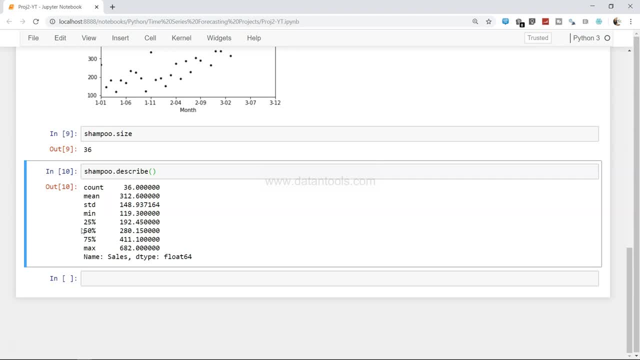 you basically the most repeated value in the column, that's, that is also. these are basically part of a measure of central tendency, which is a statistics concept. uh, when you read about it- uh, the statistics it- it all becomes pretty clear. so these are the values, and then it shows the standard. 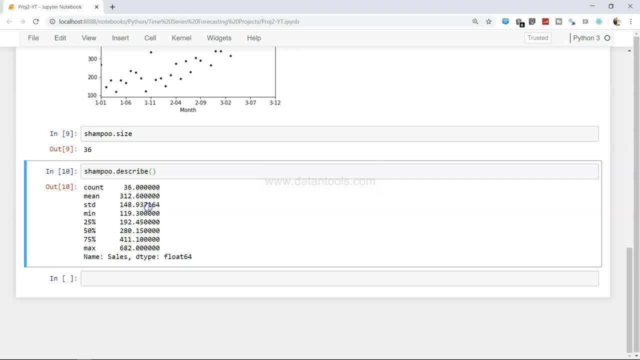 deviation. the one standard deviation is 148 and the maximum value is 682. ideally, ideally, you should be able to interpret all of this if you really want to be on the uh, data science side. what is a standard deviation over here? how you would interpret 148. what does this value basically? 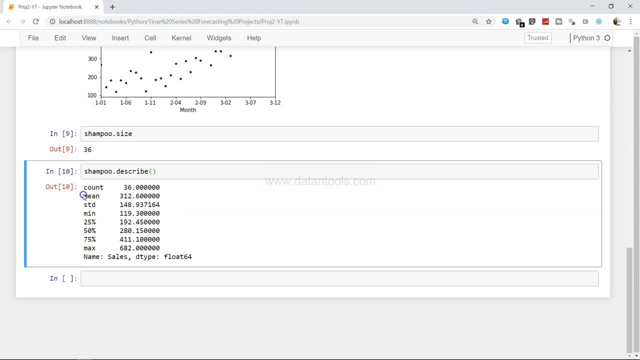 say, is 148 when it comes, like i just described, the mean and median right. so now let's go ahead and uh, first of all, uh, one of the process that we do in the from a statement, from a time series analysis, what we do豆 time. i can also introduce some details up front here and now let's go ahead, and i will. first of all, one of the ideal options for from now on. uh, we are going to go ahead and, first of all, one of the processes that, at the time series, analyst in here: stronger to be able to do something like me, and when you take care of all these are üzerine value, for we shat. 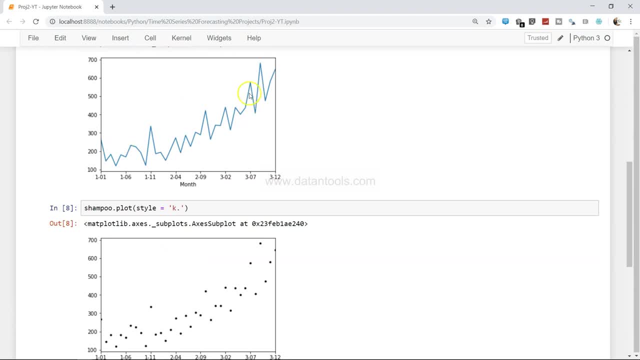 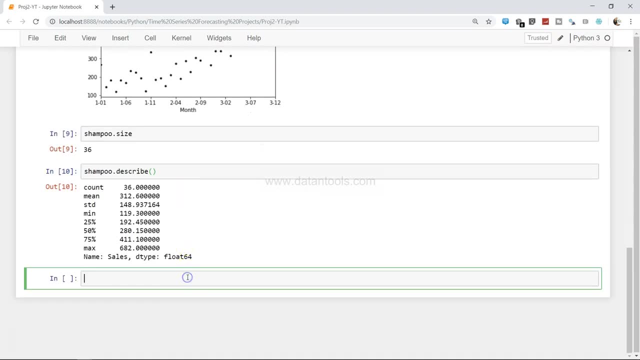 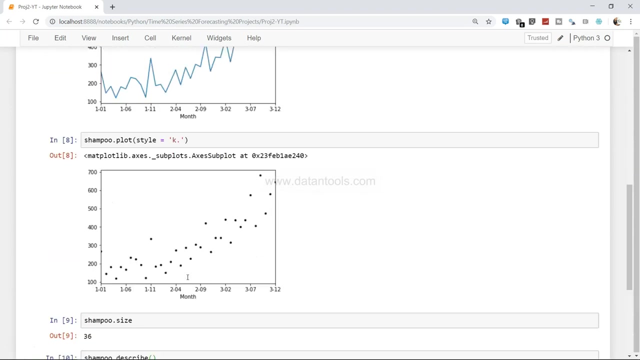 in the time series. analysis is smoothing the time series. So smoothing of time series is basically done by calculating the moving average. So what we will do is shampoo underscore. moving average is shampoo dot rolling and we will say: window equals to. So what it means is how many. first, 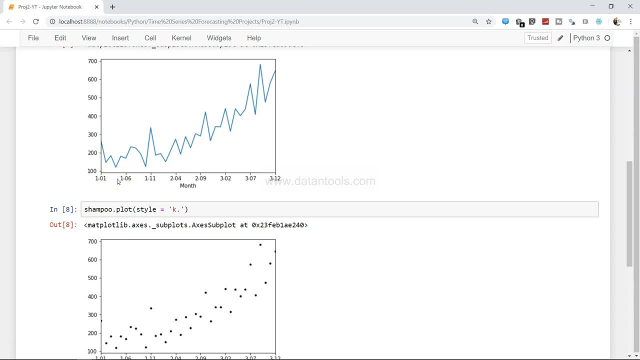 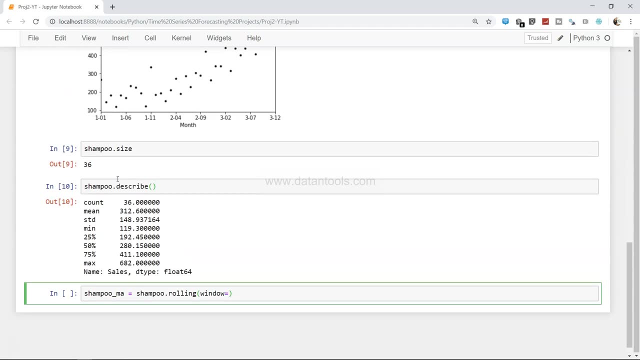 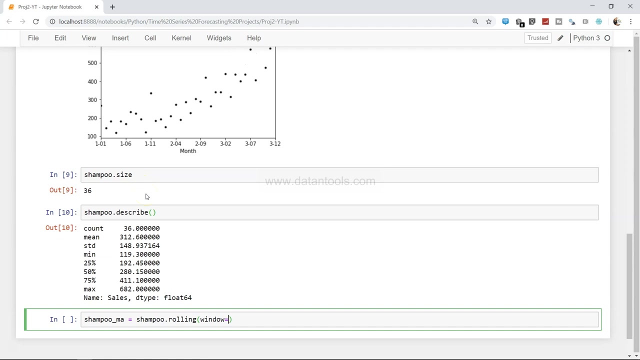 three values, five values. So for how many average values we want to take an average? I have shown this concept in my very first video on the time series. If you want you can go back and look at that. But what it basically indicates that five day moving average, six day moving. 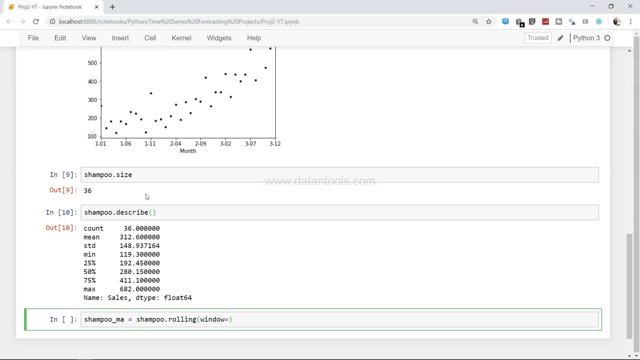 average in that first five days moving average takes into the consideration and on the fifth day you get a one value. So that means the first four value basically gone and then the value is basically starting from the fifth day. So right now I just take 10 and then 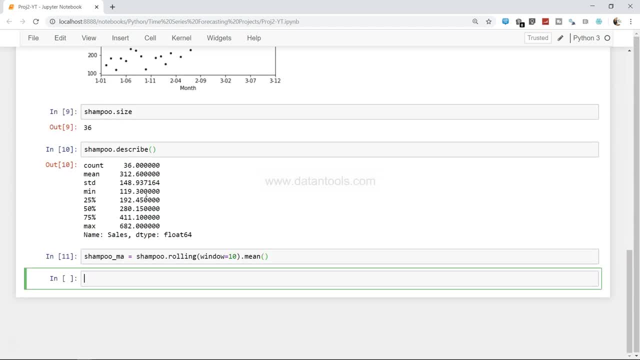 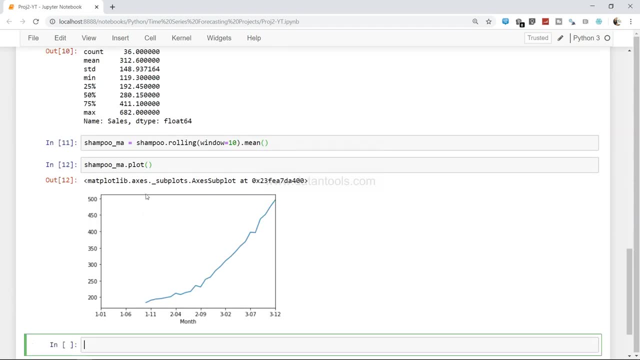 I want average. If I do that and if I plot this, You see that it is very smooth and some of the initial data point has gone and the value is starting from 111 because I used the window equals to 10.. The for the first couple of values, uh. 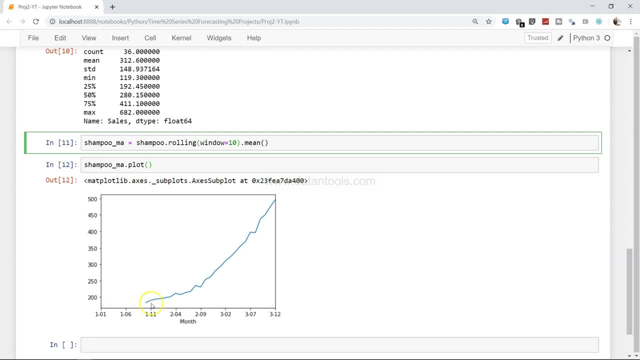 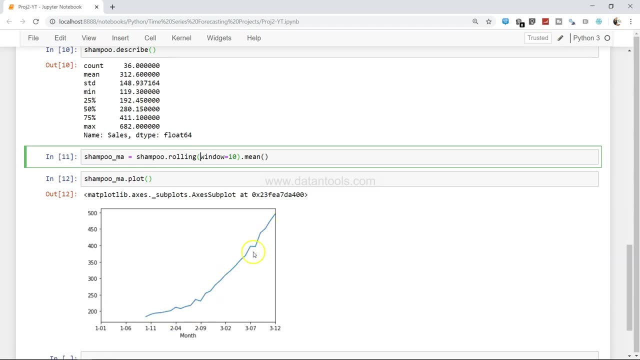 1 till 9.. 9: the value has gone, so from 10th it will be starting. 11 is here, 12, 13 and then so on and so forth. if you see, this is a very smoothed, smooth series as compared to this one. so just to understand. 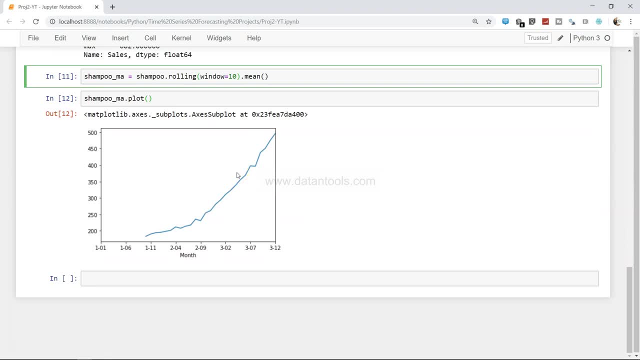 whether this series is following any trend if it is not very clearly visible. you use the moving average over here and moving average very highly used into the stock market analyst as well as in some business studies as well. but stock market analyst is the one area where I have seen that. 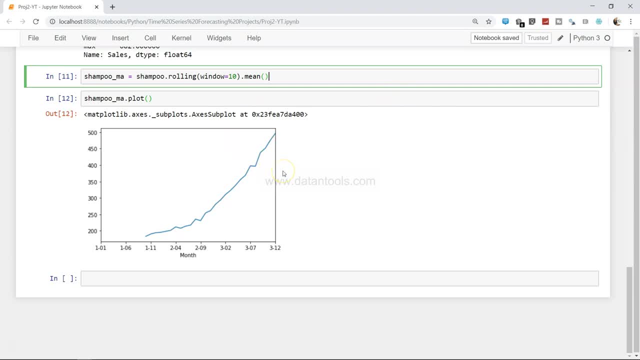 this moving average is being used a lot, a lot, okay. so with that, what we can do now is create a baseline model. so so this is just for the representation, that how you create a moving average, which is also an interview question, and the interview question is also about the the. 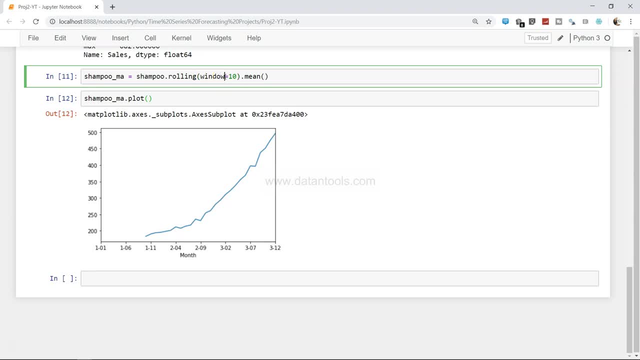 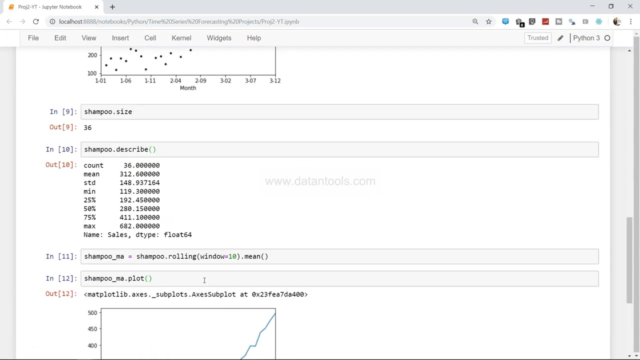 window size that we, you need to basically have, and what is the downside of having the large windows? I swear that explained that entire thing to you. now what I want is simply the creation of baseline model. so what is the baseline model? so if I just say shampoo, right, so what baseline model really? 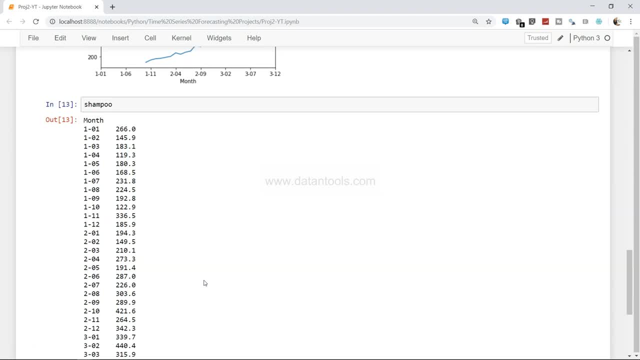 helps in the time series and it isn't to a question that what is the baseline model, if, or what is a naive model which is or what is a starting model. all of these are like common terms, that baseline knife or initial model, which is like defining your baseline. below this, if there is any model, just remove that. 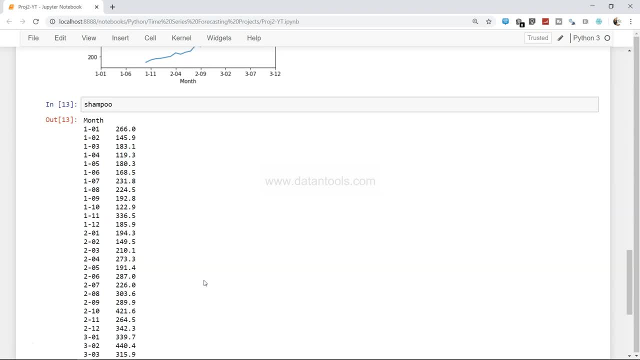 so. so the first model is like no-brainer. I mean, anybody who does not even know about data lines should be able to understand that, because if you have a baseline model, the baseline is going to be it one single base line in your baseline body. so if you are a structural engineer, you just need to. 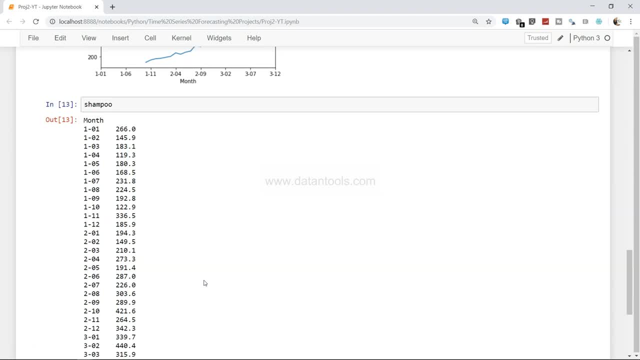 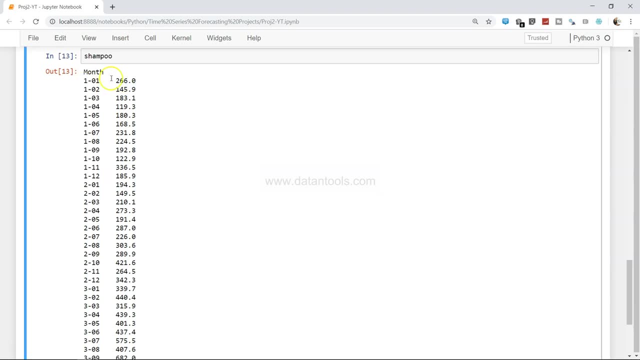 to do it and the method behind, or the assumption behind that, is that the previous value, which is this in this case, previous value, is the best reflector of the next value. so for 260 for 2nd january. so this is a second gen, this is the first gen. for 2nd january, the best reflector or 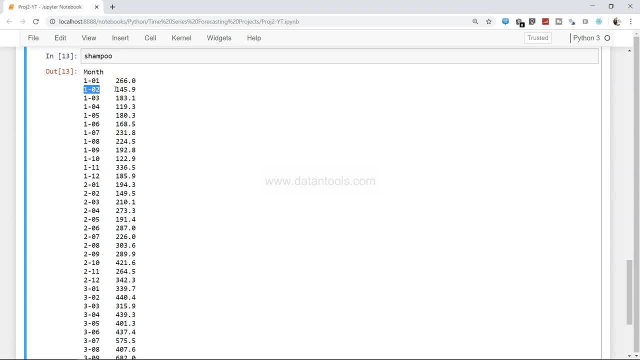 the best prediction, as per the naive model or the initial model, is the previous value. so for second, it will be once 266. for third, it will be 145. for fourth, it will be third. so what it basically assume that the previous values are related to the current value. so what we have observed last. 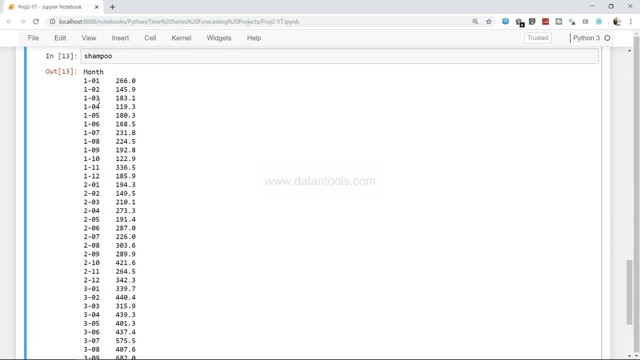 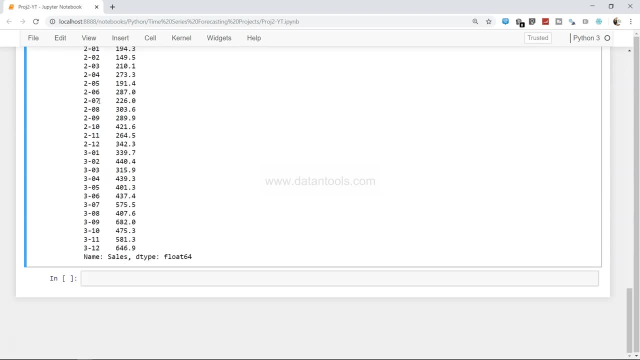 day will going to reflect also in the current day, with some more variation and with this assumption into the time series, we go ahead and create the naive model. so to do that, what i need to use is basically the shift method. shift method helps to shift the data points one point down right. so what i do is: 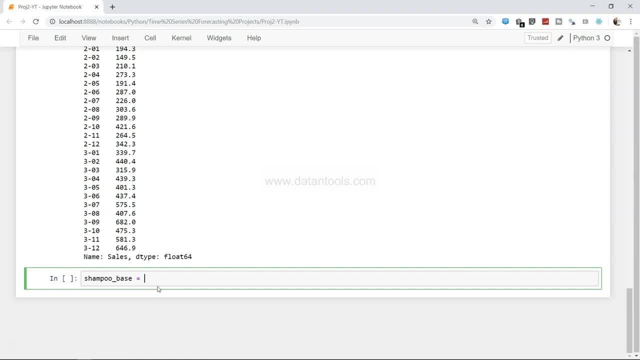 shampoo underscore base equals to: i will use some method. i will explain you: pd dot concat. because i am not going to use the pd dot concat method, because i am not going to use the pd dot to shop corner laid on the pd dot, on the pd dot convention, don't worry so. placing a head and 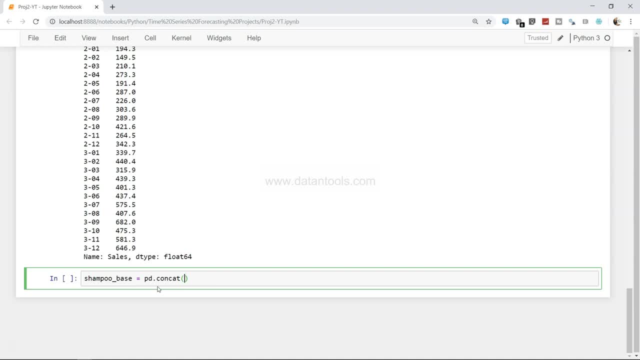 creating a separate column all together using a common technique, but i am just creating, i am concatenating as well as creating, which is a process, a little move it even further: 2016, step-by-step. so i am saying i need shampoo in this shampoo, need one column for the one, cities and 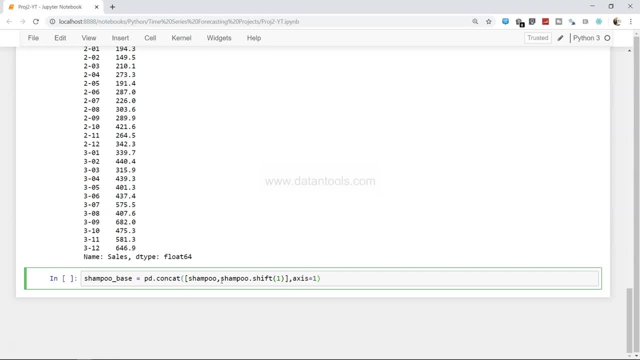 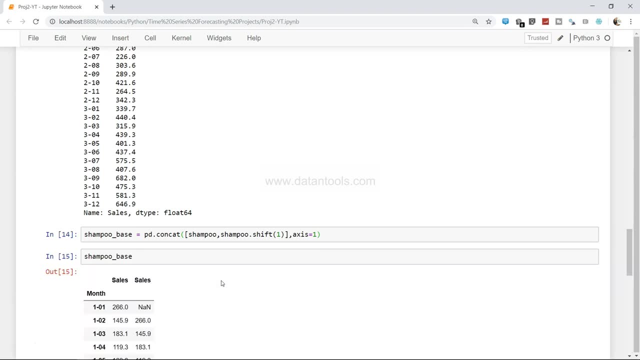 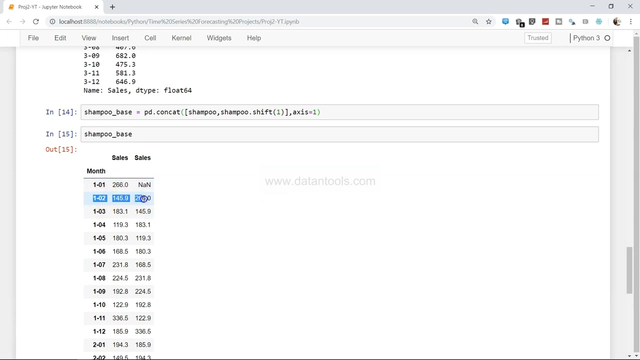 sampleshift by one. that means put the shift now in, and xs equals to one. so if i execute this, you will see that shampoo underscore base is this: sales 266, but for forecast it will be here 266. 145 is here, 183 is here. so the structure of our 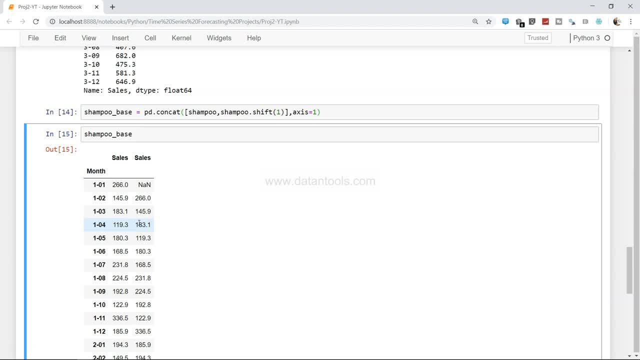 baseline model is created or the naive model is created. however, if you know that you should not have this particular value, which is a missing value in this case, it gives an error when you evaluate the error metric. so so, whenever we produce model, we need to remove these values. 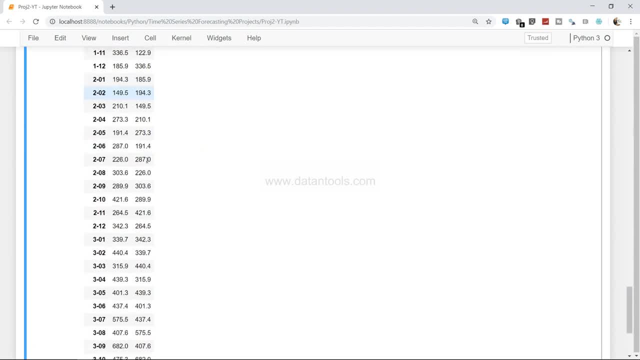 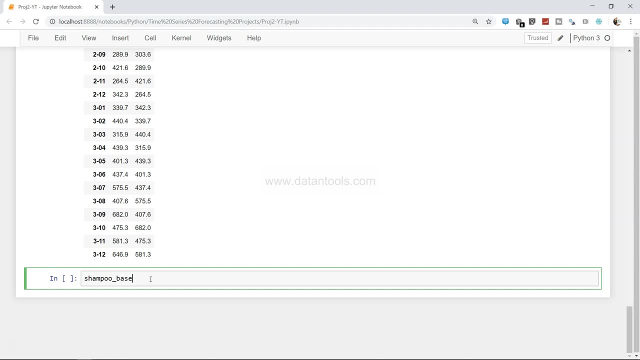 and before that, we need to give the names to these two, right? so we need to rename the column. so how you rename the column again for beginners, you need to give the names to these two, right? so we need to rename the column again for beginners. it is an interview question related to the uh data manipulation. so shampoo, dot, base columns- what? 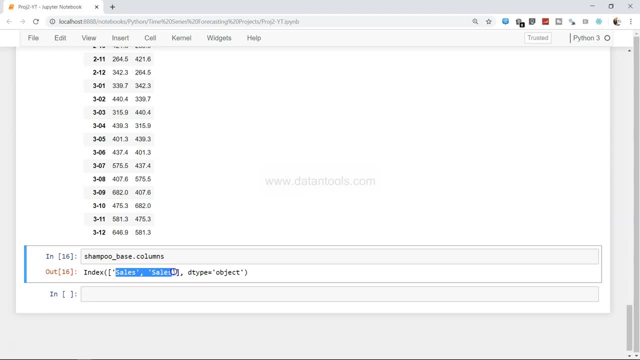 what happens when you execute this. it gives you the column names like this: so what i'm doing is i'm following the same methodology. equals to. within the bracket, i will just specify the new name over here. that is it saying actual sales. so just to make you very, very simple, that what i'm 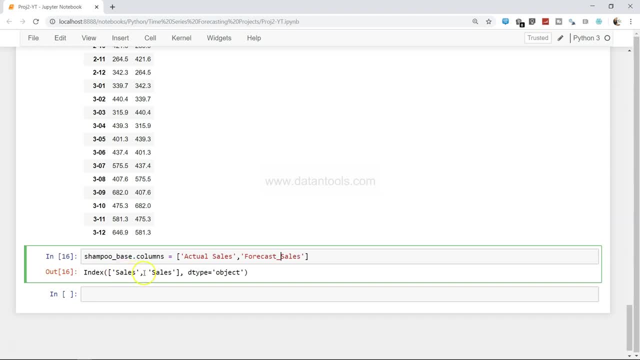 doing and how it is going to work is- i'm going to give you the name of the column and i'm going to give you the name of the column and i'm going to give you the name of the column and i'm going to- is reflecting. so this is what the representation it needs and that's the representation i have. 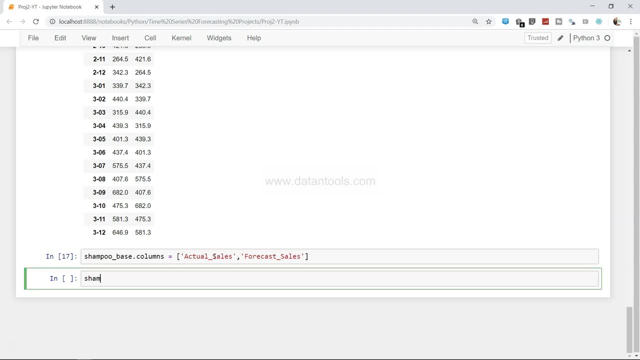 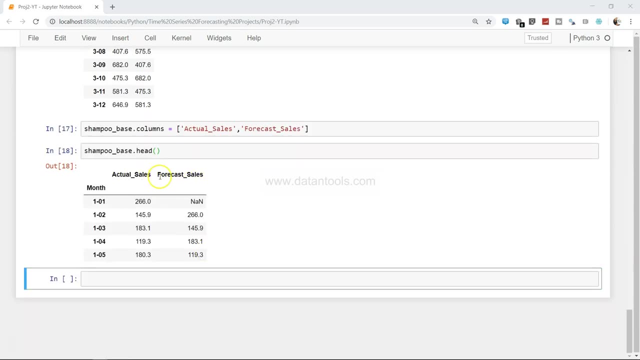 given over here if i execute this and again say shampoo, underscore, base dot hat. so actual sales, forecast sales, all right. so now we have renamed the column, the next thing is dropping this value, and to do that the method is: remember this. this comes very frequently. drop any if you do that. 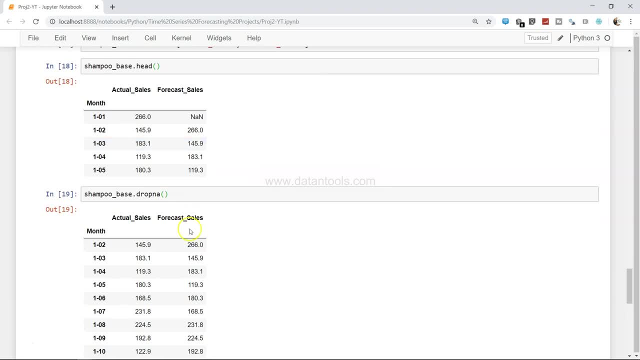 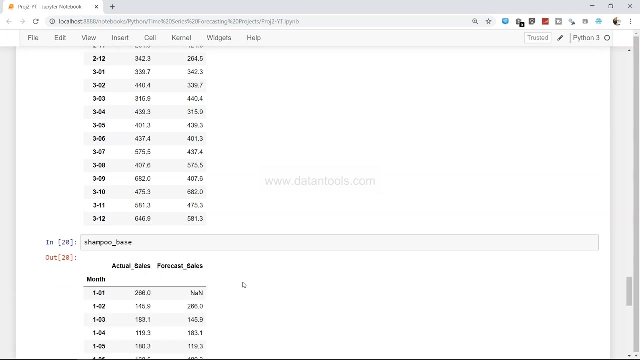 if i do that, what happens? value is dropped right, but there is a catch over here. first of all, remember the method: drop any, drop any, is a method that you use to drop the nan or the missing values wherever it presents. so it removes the entire row, if you see. but if you see shampoo, underscore base. 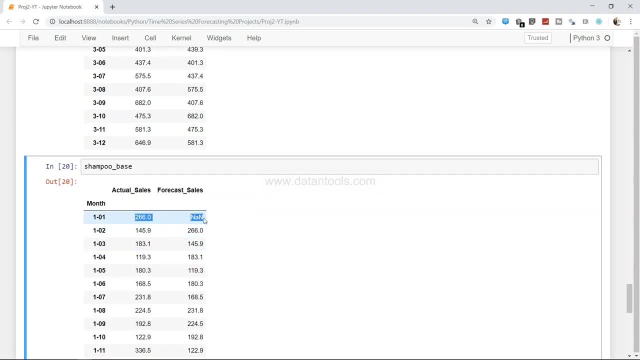 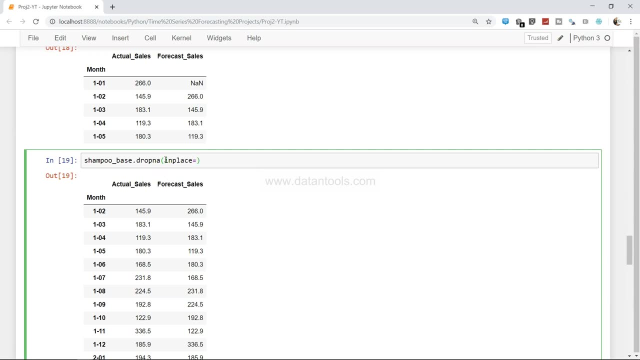 the problem is the missing value has come back right, so what i'm going to do is i'm going to remove this value. so what you need is basically a parameter over here. in this method, which is in place equals to true, so this makes sure that whatever changes, changes is basically dropping. 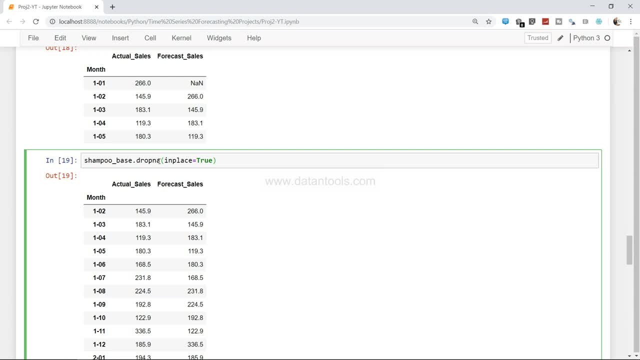 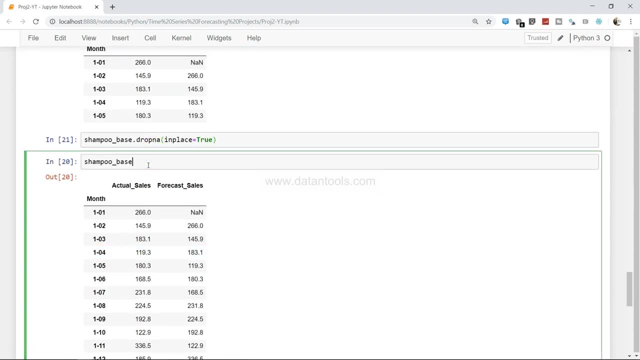 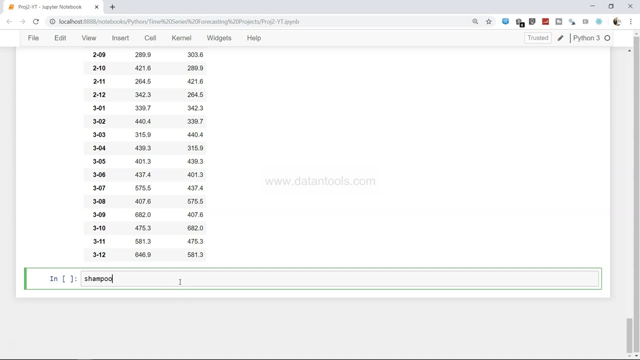 the na value is saved or has become part of the data set. so if i execute this- and now i am here- shampoo base, if you see the value is removed. if you want to check it again in a new column- shampoo underscore, base dot head. you don't have that value, so this way you make sure that you have the 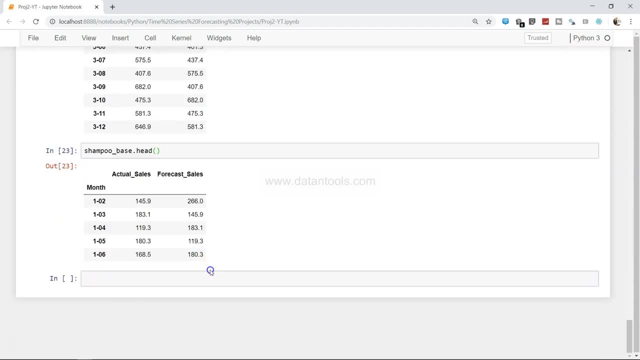 proper parameters and everything present over here which is responsible for making sure that your data set is, that your data set is properly made for the baseline model. now let's go ahead and import the mean squared error metric and the numpy array for the calculation of error between the actual and forecast sales. so from sk learn. 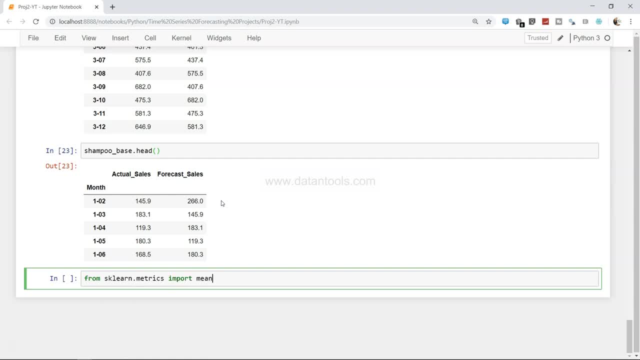 dot matrix, import mean squared s, q, u, a, r squared error and then import numpy as np. so y mean squared error simply gives us the mean squared error error. but the problem is it is squared so it cannot be. we cannot interpret it in the same term. so to remove the square what we need to use is np dot sqrt, the square root method, which will 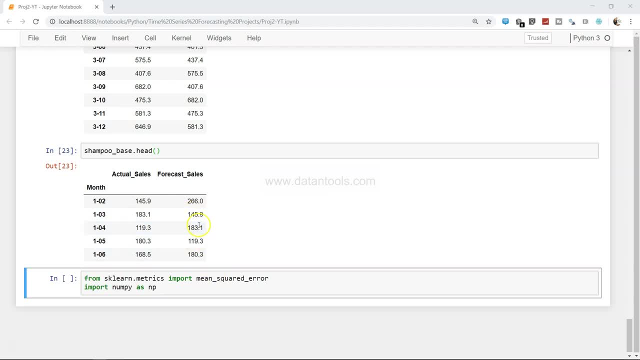 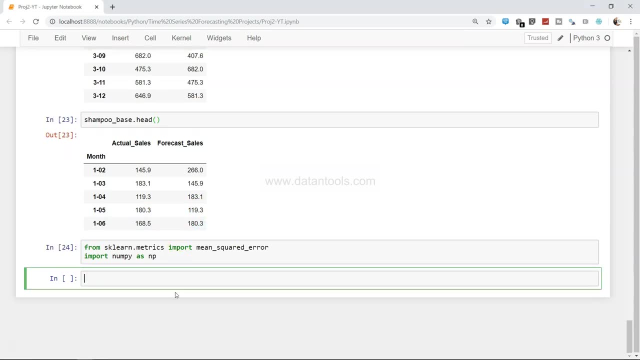 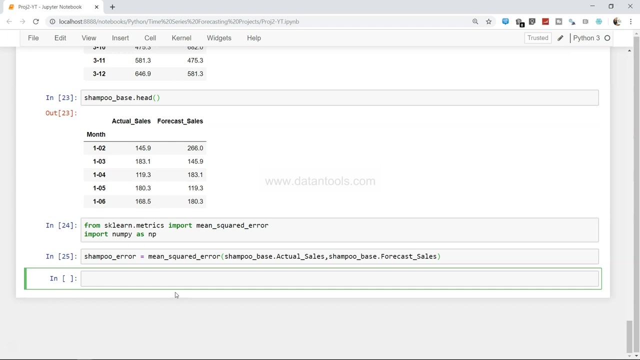 keep it in the form which is similar to this value or in the same matrix system in which this value is being calculated. so let's go ahead and execute this and after that we have shampoo underscore error, mean squared error. shampoo base dot: actual sales. shampoo base dot- forecast sales. 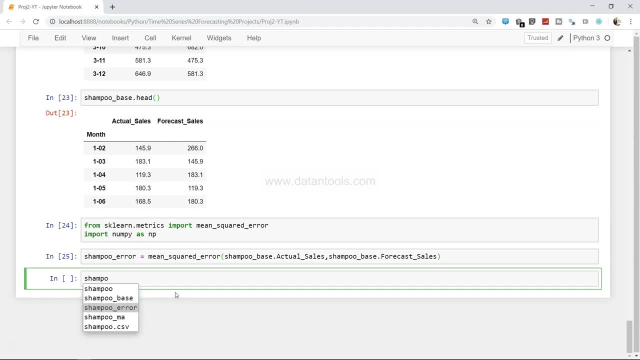 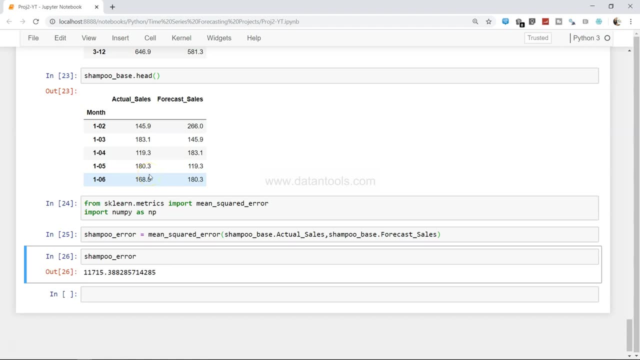 right. so if we see shampoo error, so the value is 11715, which is definitely not anywhere related to the matrix system that this particular you, this particular data set follows. it may be in thousands or it may be in millions, who knows, but this is definitely not following this. so what we need is np, dot, sqrt and then the shampoo error and 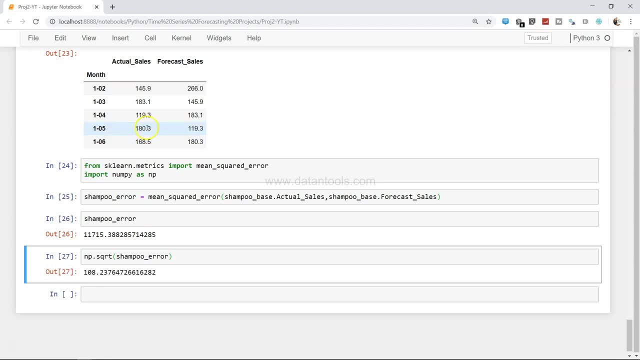 this is like 108. so now the value, you can relate it with this particular metric, which is in the similar lines, so you can interpret it as per the. you know the math, the metric that your data is following. all right, so that's now. what we can do is we can create different types of models, for example there: 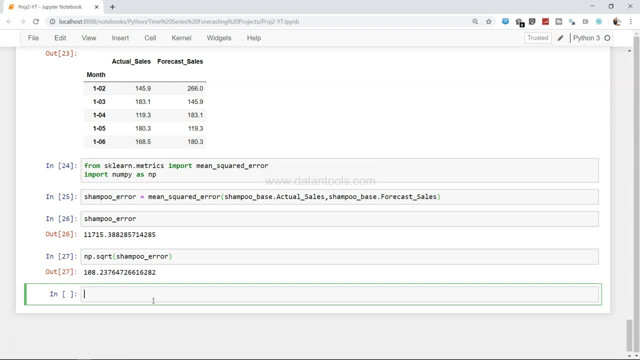 is a moving average model. there is an auto regressive model. uh, there is differencing that you can do to make the series stationary and whatnot. so we're going to do a amongst the created models. but at the end of the day, if you will see most of the practitioner, the real time, those who really work, basically use 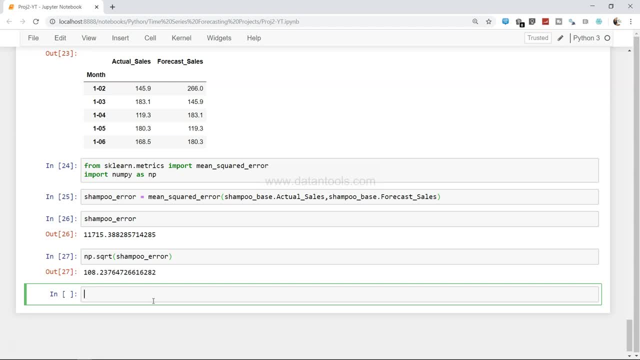 the arima method, which is auto, regressive, integrated, moving average. so for it. so it contains everything it. it contains autoregressive, it is integrated, it is moving average. all of that is part of one, one single model. so i just don't want to use and, uh, you know, make this video very- 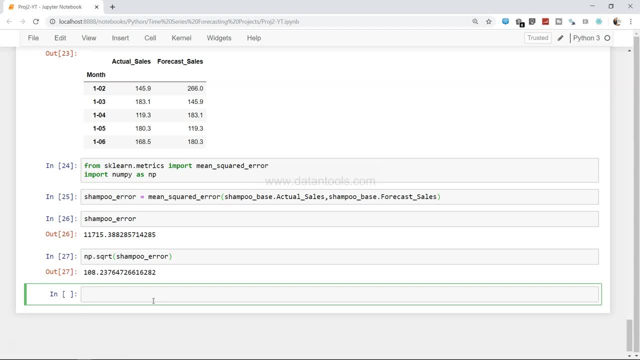 very long, but just want to make it concise so that we focus on the main topic, which is arima and within arima. if you say you can create an autoregressive model, how you just specify the term or the parameter for ar, which i'll show you. for example, arima is like this: p, d and q. so in 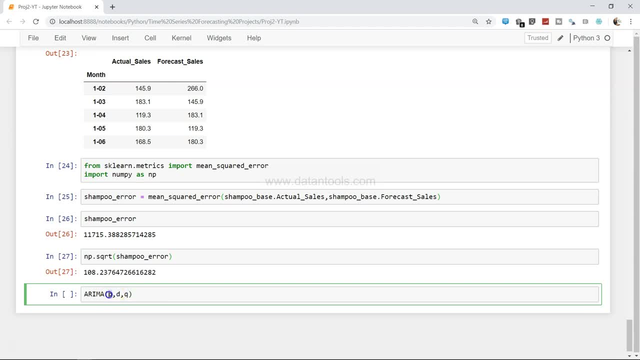 this: you have p. the parameter p is nothing but the autoregressive. so let's say, if we have the model arima, 2 comma, 0 comma 0, that means only the p term is specified, so it is an autoregressive model. so why should i go ahead and create a separate autoregressive model? or if i say 0 comma 0, 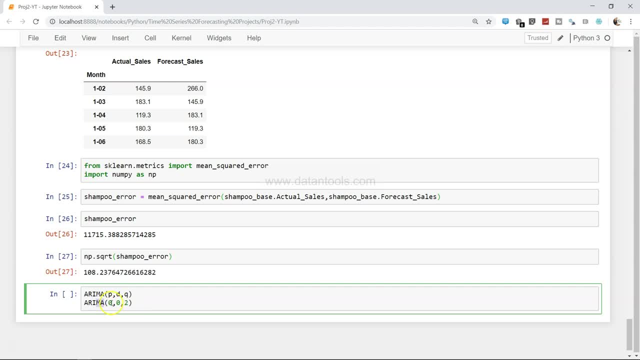 comma 2, then it is a ma model, moving average model, because we are not considering the last two. so so if if you are a very, very experienced practitioner and coming into the python, this is the way you can do it. you don't have to experiment and know a lot of different values within the arima. you can basically create either autoregressive, 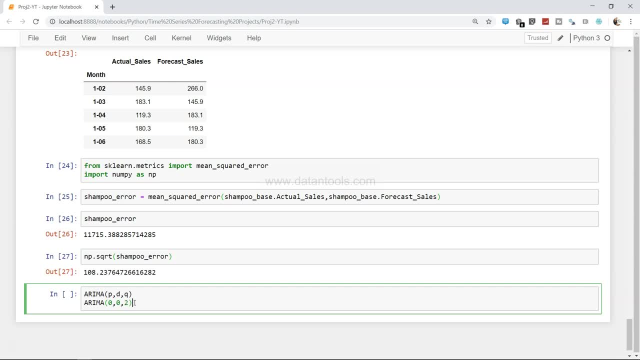 or the moving average, or a combination of everything which i will going to do in just couple of minutes. so autoregressive is, we need to calculate the autoregressive and the moving average term by having the acf and pacf. so just remember, pacf is to evaluate the parameter for. 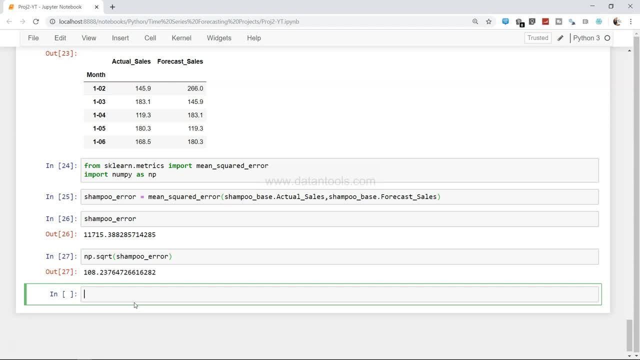 p, which is autoregressive, and acf curve is for moving average. okay, so let's go ahead and first of all get the stats models, dot graphics, dot tsa plots, import plot underscore acf and plot underscore ph, cf. so from the from this term, just remember, pacf is for p and then next another one which is without. 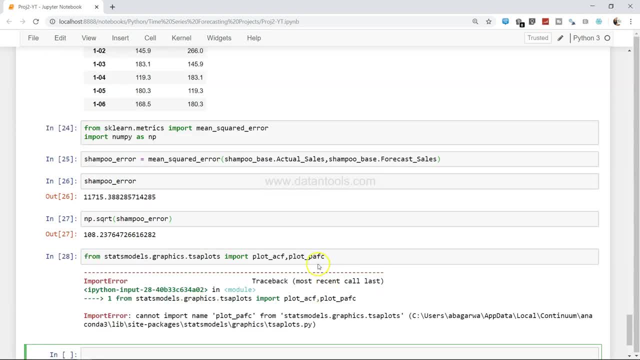 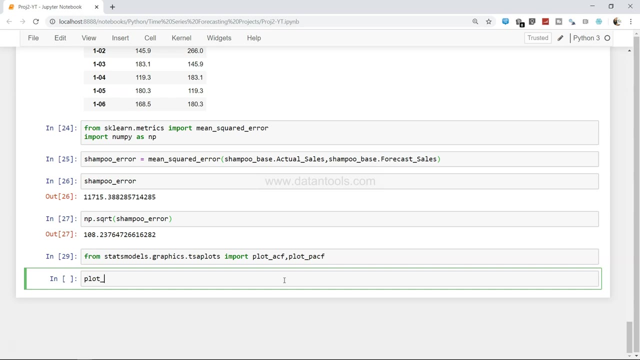 p is for q. that's how i remember it. if, if i. if it is confusing like acf and the pacf, all right, pacf, i mentioned pafc. that's why it gave the error right. so what i'll do is plot underscore acf to c. 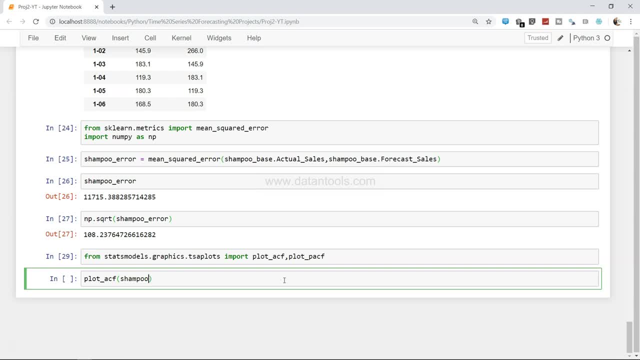 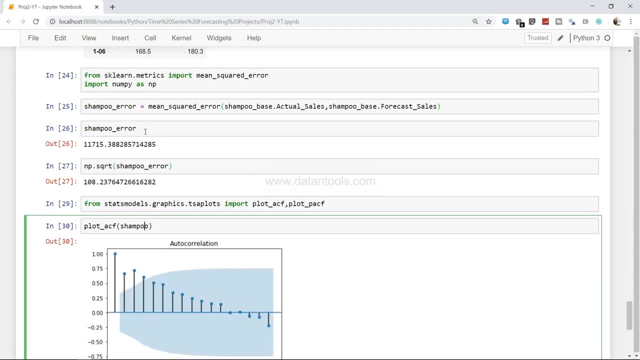 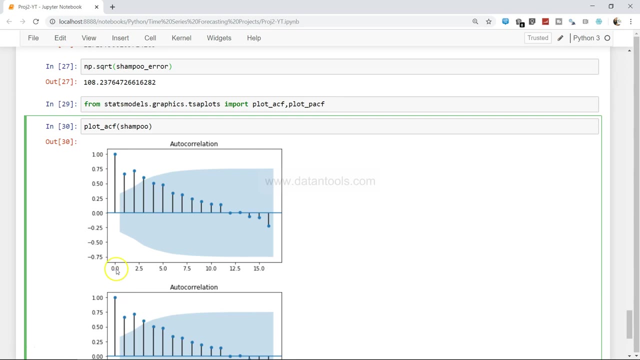 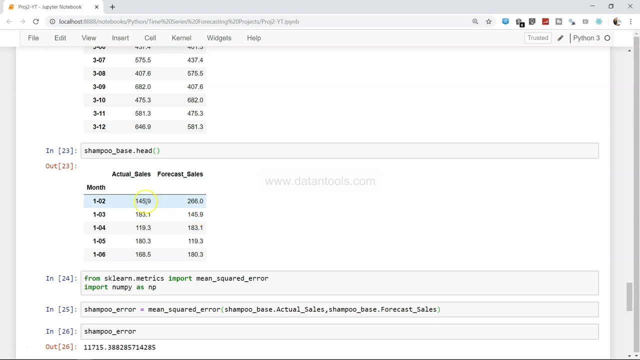 the q term and that is shampoo data set. i'm picking up the entire data set that i created previously, but not from the base model. so what it has is basically at the term zero. that means this value is equal to this value. that's what zero basically mean me. or if i just go back just for a better in. 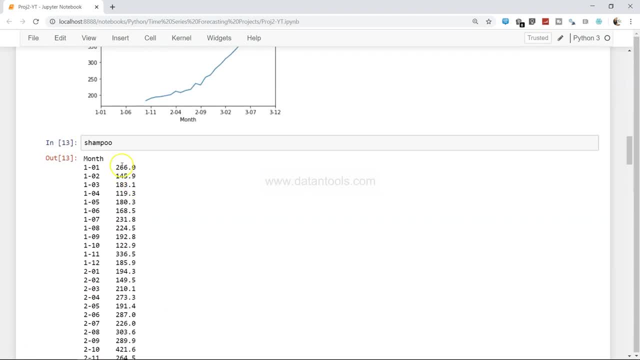 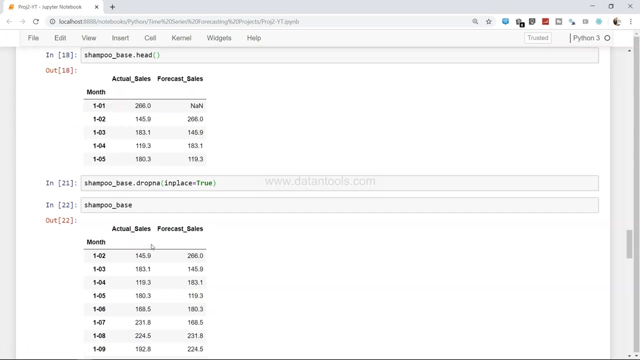 in view for you. sorry about that. what it basically has at zero term is to 266, equals to 266. then what is the correlation between them? and at the one term, what is the correlation between these two? so that's what it basically calculates: the correlation with the existing, the one previous term, the. 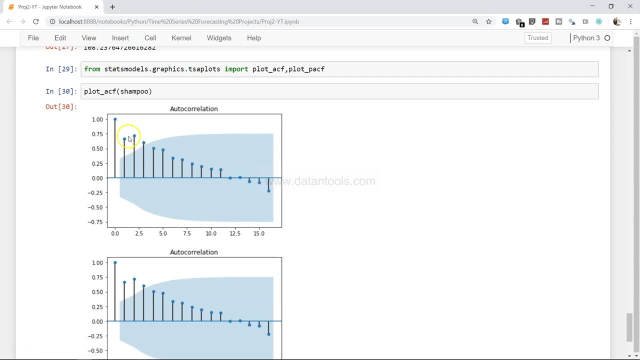 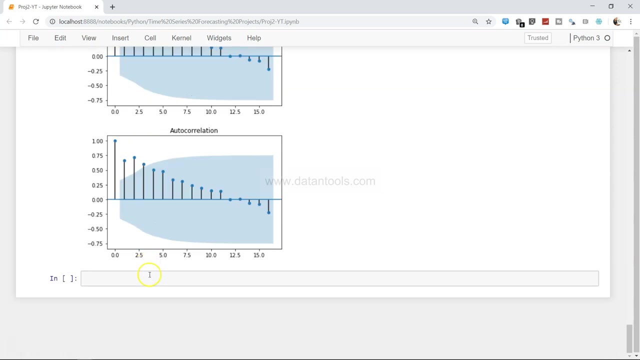 second previous term, the third previous term. so over here it shows that the third previous term, the correlation, is going below the range or the critical range. so when up till what value you have out of this critical range, you consider that and uh, so, for in this case the q will be the three, zero, one, two, three. so q or q is. 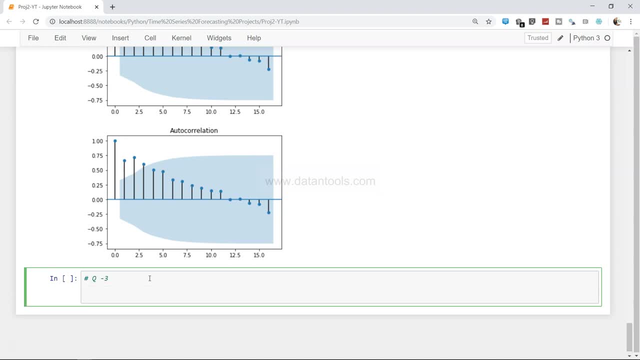 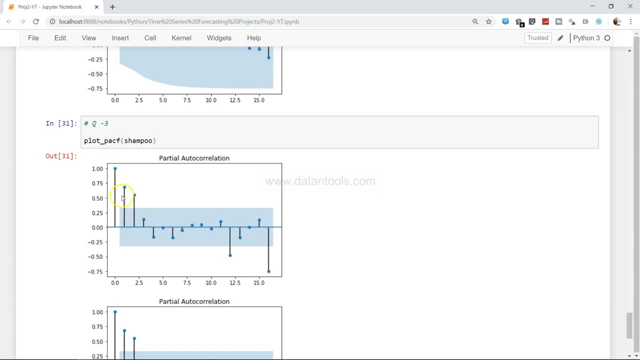 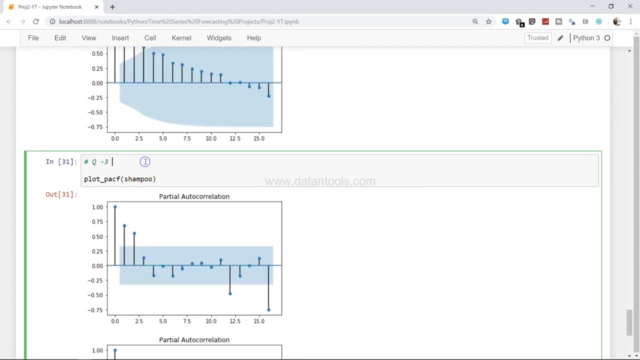 hash q is three is something what we figured it out. now what i do is plot underscore pacf and shampoo and in this case after the second term, 0, 1, 2.. so you have p as 2. now what we need is basically differencing term d. 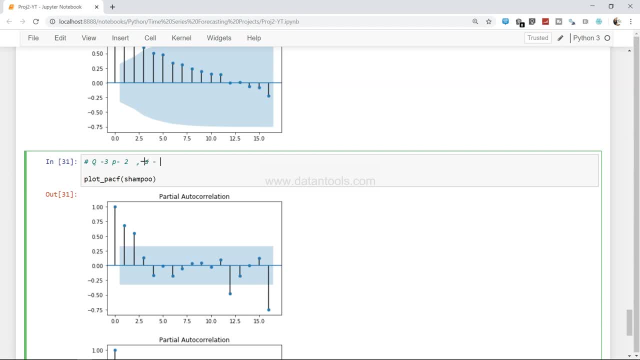 to make the series stationary. i'm sorry, all right. so usually it is between 0 to 2, ok, so we will experiment it between 0 to 2. maybe 1 is is sufficient, but we can even try it with two, okay. so this is basically the number of rotations that we are going to note in this one. so I do not know that is sp or D as small buter degrees, and they divide one by 6. okay, so 501 equals to say, actually it is pause relationship. i want to to me to be okay. so usually it is between zero to two. so we will experiment it between zero to two. maybe one is is sufficient, but we can even try it with two, okay, so 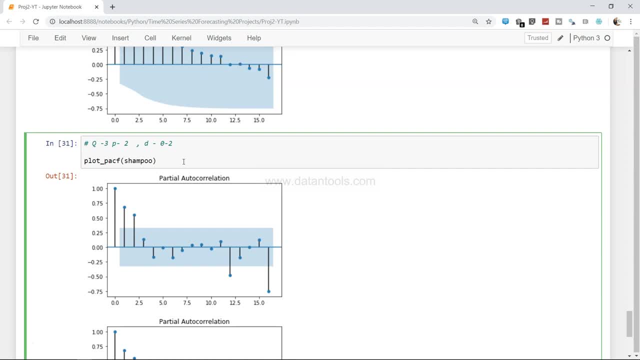 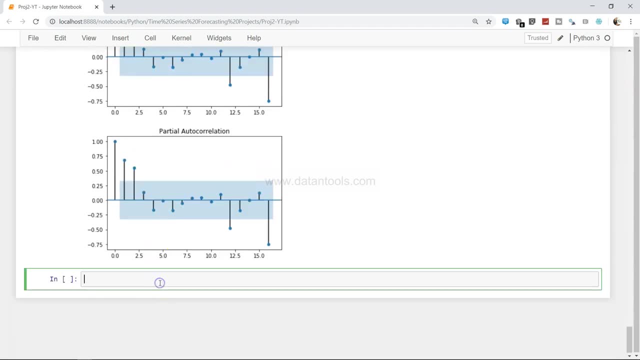 what it does is make the series stationary by removing the trend and the seasonality factor, which is how, which helps us in doing the better prediction. all right, so now let's go ahead and import the arima model from the stats model, so from stats models dot tsa time series analysis. 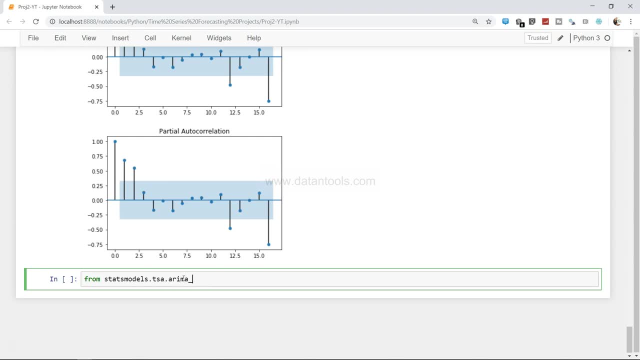 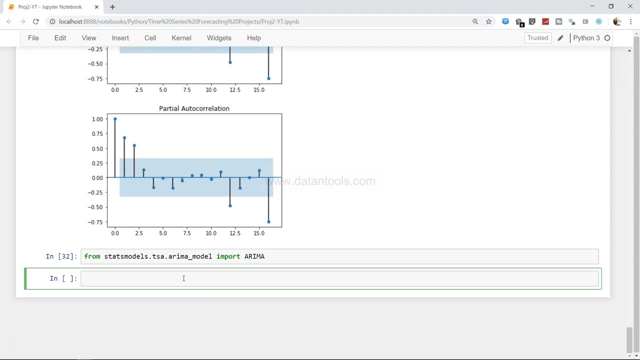 dot arima underscore model. um, what do you have is arima, execute this and i'll just create the train and test. so train is shampoo 0 to 25 and shampoo score test is basically shampoo 25 to 36. so it will take the value from 0 to 24 and you need to tell me why, because this is an 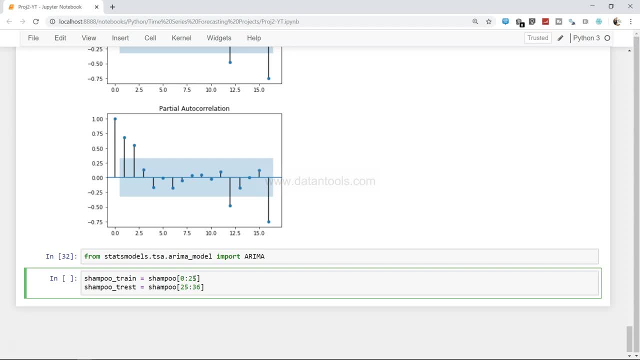 interview question and i already explained in one of my previous video- if you have not followed it. so if you're not followed it, go ahead and see that- what i just wanted to complete the sentence. all right, so first 25, uh, 24 values. i have taken over here rest of the values in this. 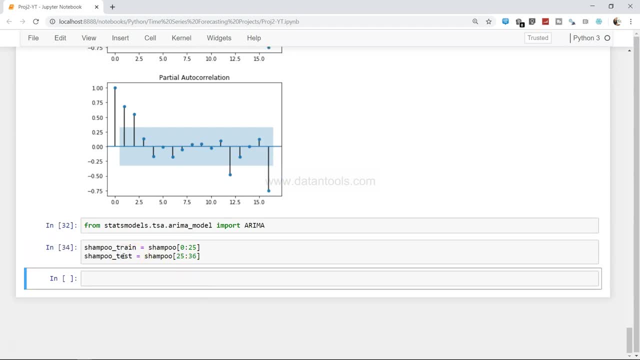 and if i execute sorry test, if i go ahead and execute this, you'll see that i have taken over here and i have taken over the rest of the values in this. and i have taken over the rest of the values in this and i have taken over the rest of the values in this. 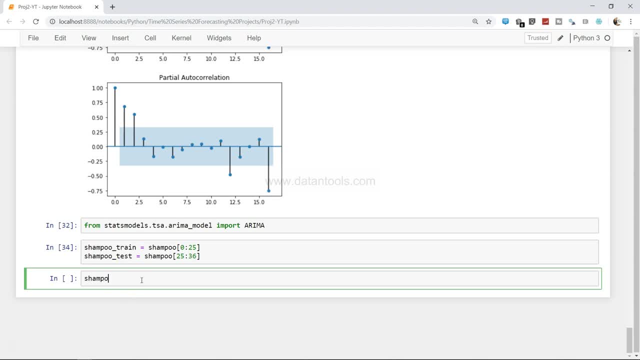 you get the train and test data set, so i'll just create the model which is arima using the train. so train and test why we create it, if that's what it is going in your mind, just to make sure that when we evaluate our model, we have some unseen data which we are 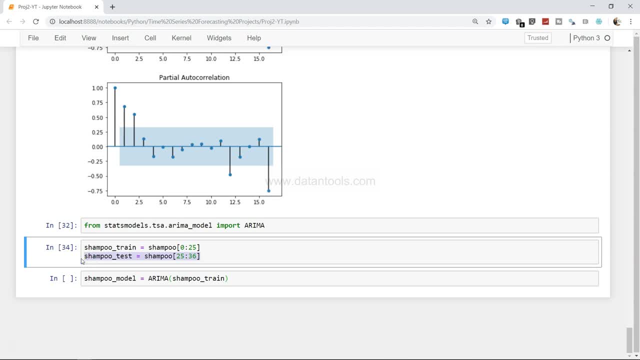 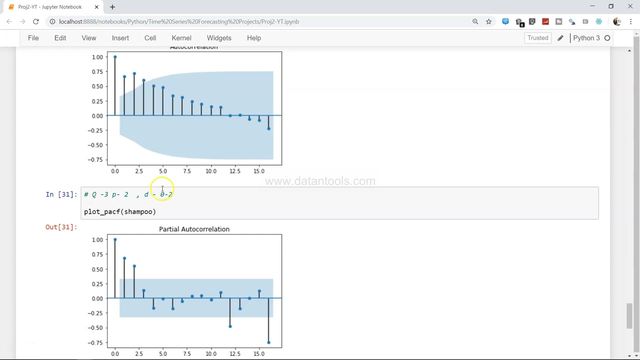 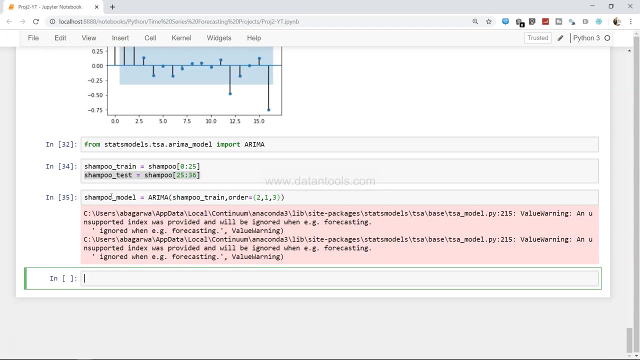 keeping it in the test for the calculation of error metric, which is a best practice. so shampoo underscore. train order. order is what we need to specify: three, sorry. two, one, three. let's try with that. sometimes it gives error, but not an issue. two, one, three. so it's just a warning. for now we can just go ahead and ignore that and 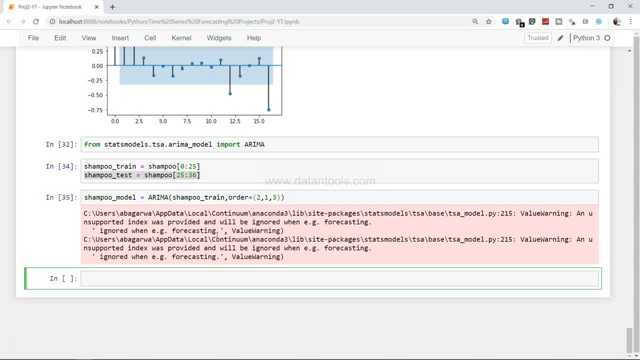 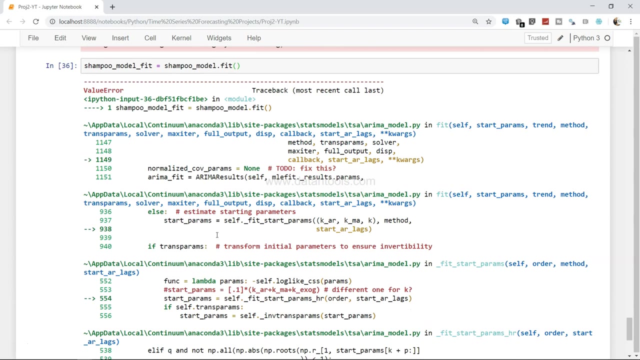 uh, now what we have is the shampoo model. we need to fit it. that's a part of the process. once the model is created, you need to fit using the shampoo underscore model dot fit. you should include invertibility. choose a different model order. so it's not. 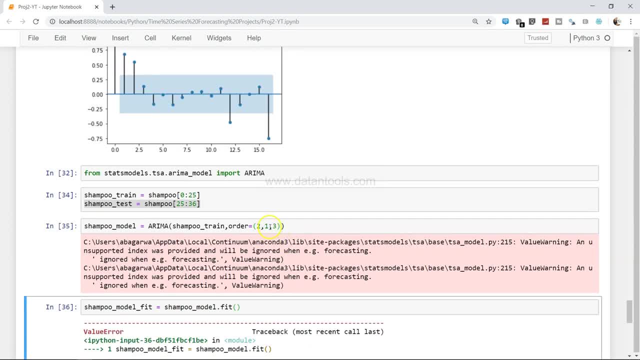 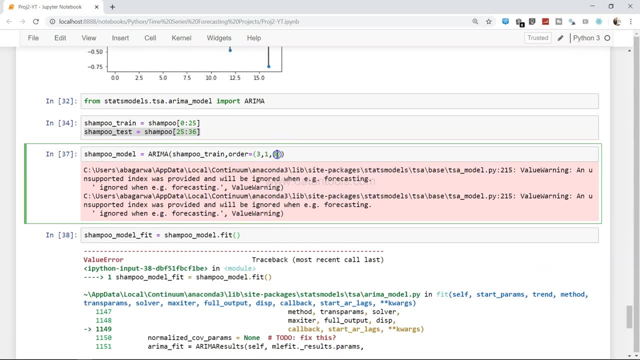 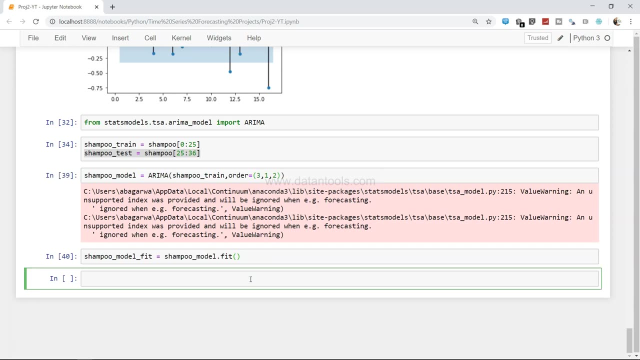 uh allowing you to use this particular model. so what i'll do is i'll use three one three. no three one two. so i'll use three one three. so let me try that. yeah, in that case it has worked. so it it gives, based on how, uh arima's. 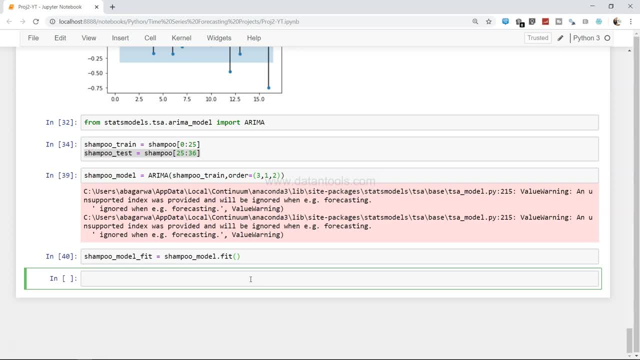 dependencies are on the model creation. when you fit the data, it basically gives the warning, like in this case, which says that whatever order that we have specified is not, uh, consistent. we need to have the consistency generally. in the case of arima, we need to make sure. 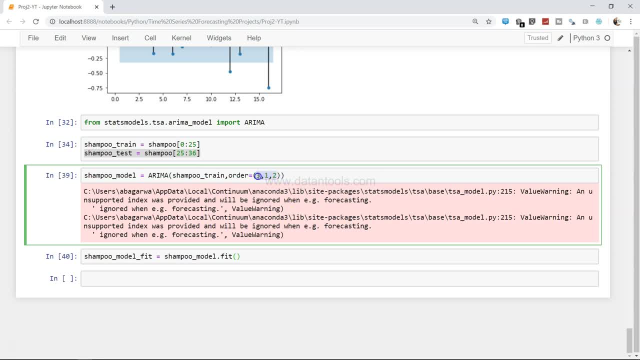 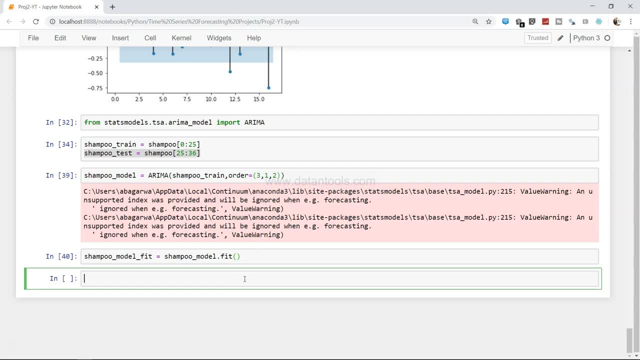 make sure that. We need to make sure that by making clear stains after flicking in all the building coordinder we'll get that description and we can view the setup and adjust the and adjust the SW Studien, undefined. So back when you make the encorei if it was just cheated. Maybe it won't be that244-57.. So we need to just tune out cattle, a couple of orders to get the right fit, okay, and i will tell you the model tuning also, which is an automated way of doing the things, so don't worry about this. all right, so once we have this, we can have the, the Forecast, so shampoo Madder spilled for it. and before i do the form it, because i'll just tell you one more thing, which is a kite information criteria, which is used to see if mynerFP4 and when i have two, 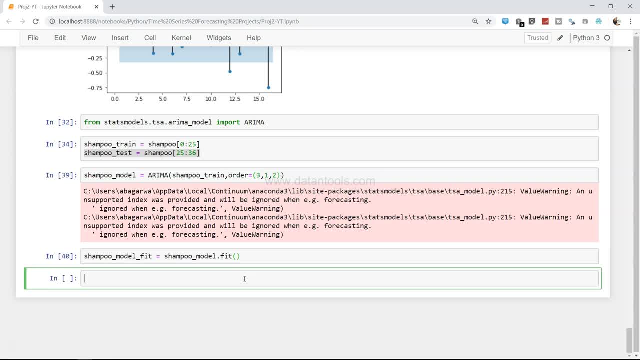 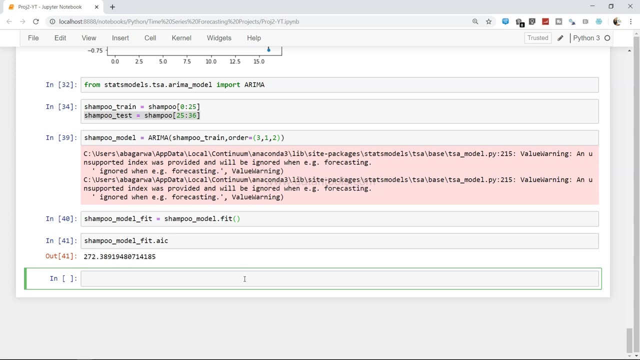 how good the model is once you fit it, and lesser the value, better the model. shampoo underscore- sorry, shampoo underscore model fit dot AIC 272. not an issue, we'll just go ahead and test it. so now, shampoo underscore forecast. that means create the error metric for a cast equals to shampoo. model fit dot for a. 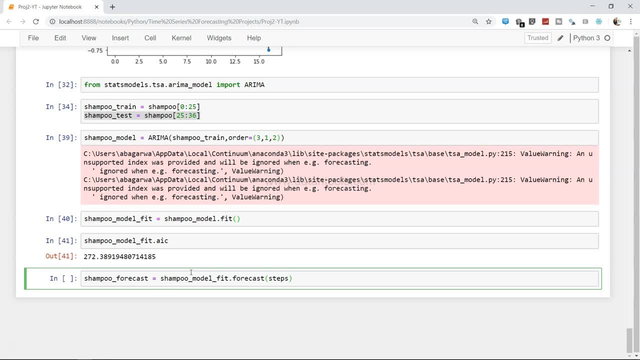 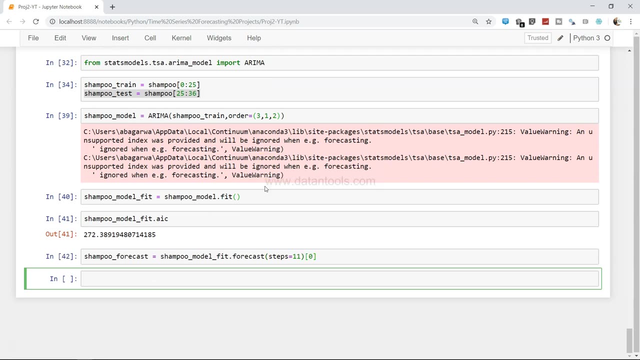 cast and steps equals to. so we took 0 to 25, and that should be the next 11 values, if I'm not wrong, and 0. all right, so it has created. so 0 is basically contains the actual forecast value. it has like two, three. 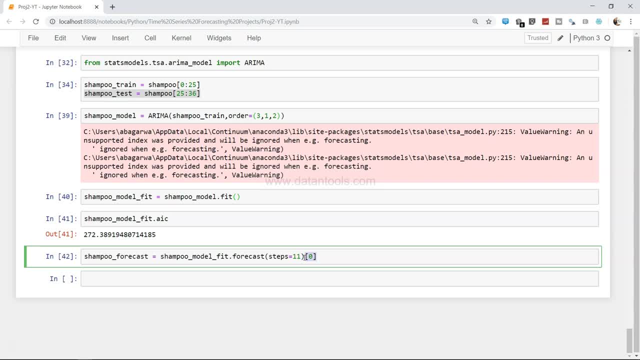 different arrays, which has like residuals and couple of other things. so what we can do is now and P dot sqrt, just take the square root of the mean squared error. I explained you already about this: shampoo underscore test. shampoo underscore for a cast. so first you will see the observed values or the. 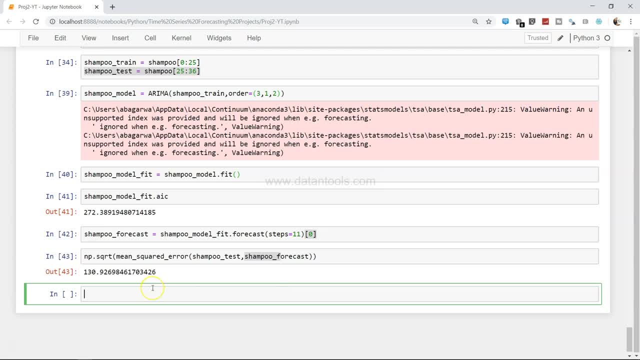 unseen values and then for a cast value. if I go ahead and execute this, what I get is the 130 is the error rate. so 130, which which I got as part of the error that my this Arima model contains, I need to test it against my baseline model whether this model is better than 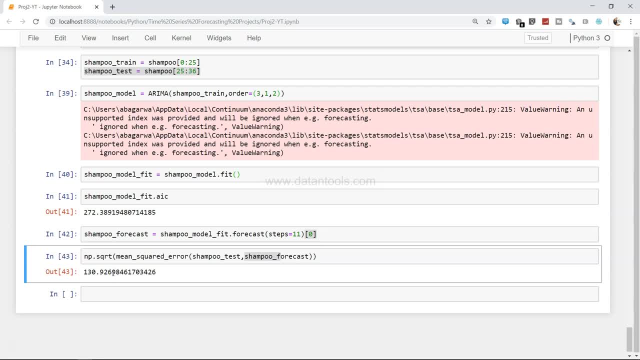 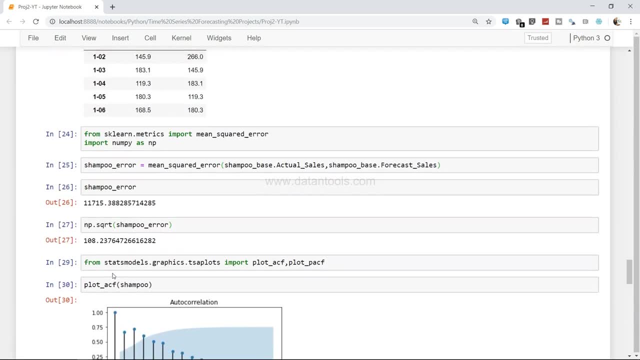 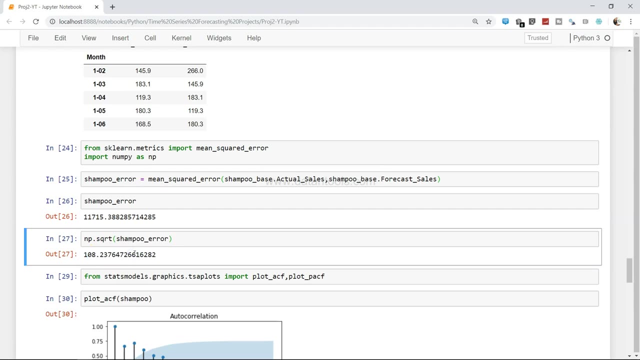 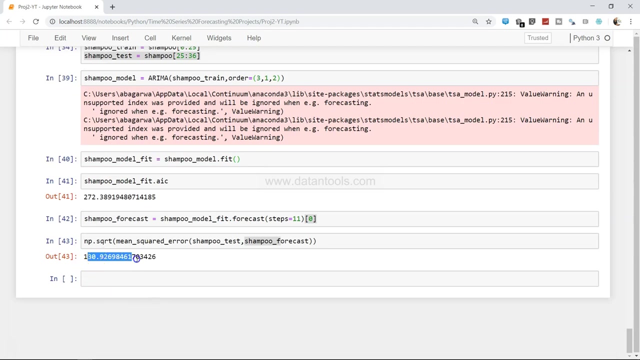 the baseline model. if it is not, I will not accept this. if it is better than the Arima that model, then I will accept that. so over here, if you see, the error is around hundred and eight. so yeah, so even the baseline model is working much better than the Arima method. over here, that: 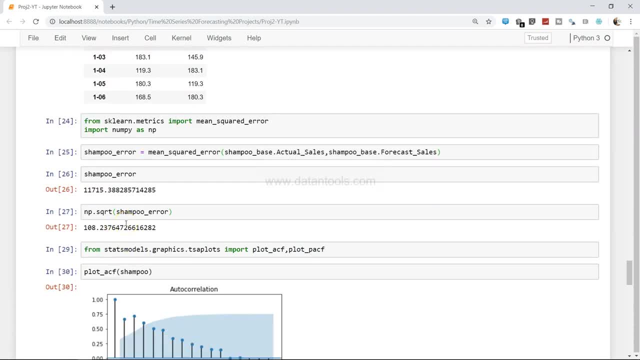 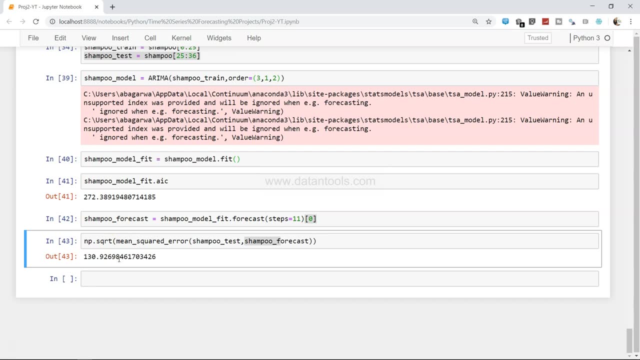 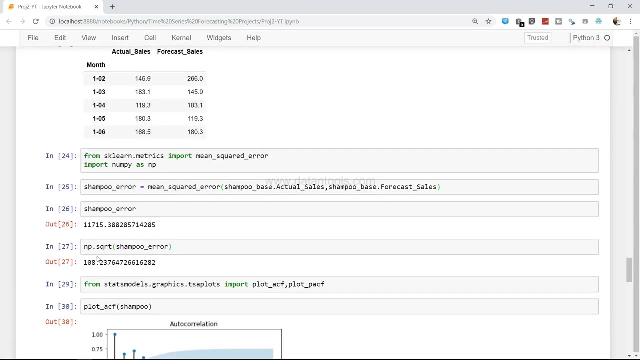 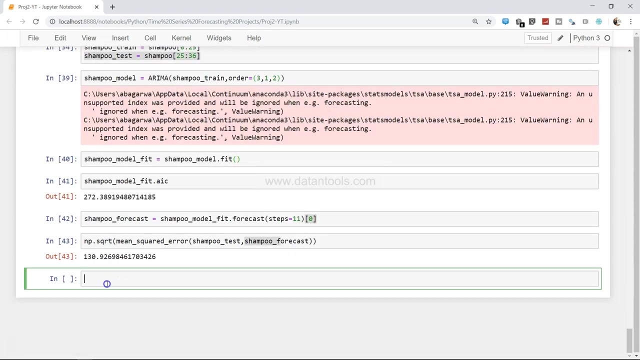 shows that our baseline model is is much better when it comes to doing the prediction than our Arima model. right, because the value that we got is 130 and and value way here we got is hundred and 108 where it is hundred and eight. okay, so this way you basically identifies whether you can accept the 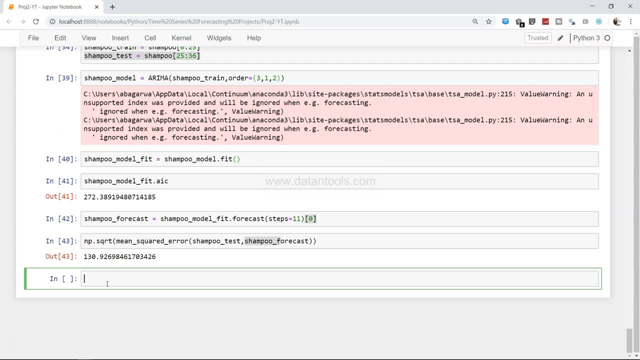 model or don't. obviously, you can tune the parameters and all, and which is basically the next thing which I can tell you. so what I need to do is is in that cases we need to specify p and the score. values equals to range in which the offset of values is same but the value is not. Его fear free. and Ulitsady values equals also pathetic. so right now, path in the healthcareSearch is that there is is something in the name of values três y Power-CustomizePlatin buttons. with that one will answer. this provides the sampling. and values and whether you accept the model automatically will take a disqualified parentheses and that Hybrid wird. es was a fundamental advantage in this model, which is basically the next thing which I can tell you. so what I need to do is is: in that case, is we need to? 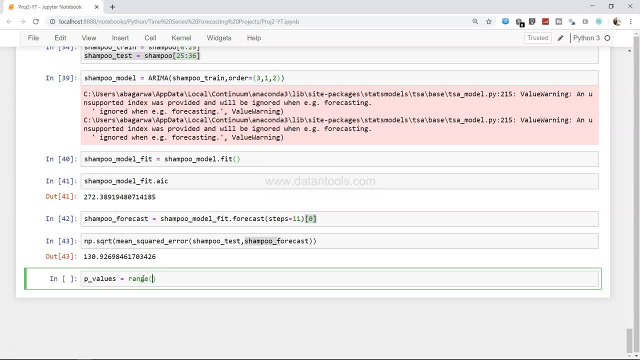 specify p underscore values equals to range, in which range you want to evaluate the p-value. that means 0, 1, 2, 3, 4. what is that value? so let's say we want to experiment between 0 to 5 the values between the range 0 to 3 and Q values. we 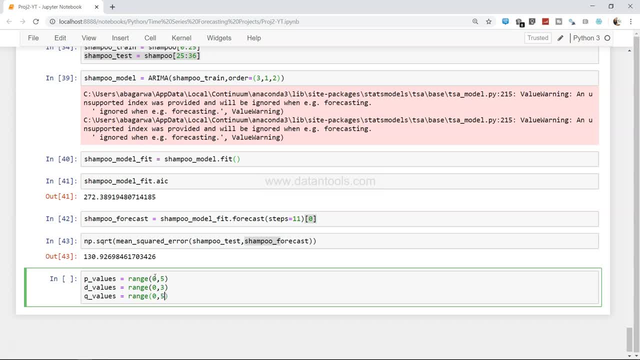 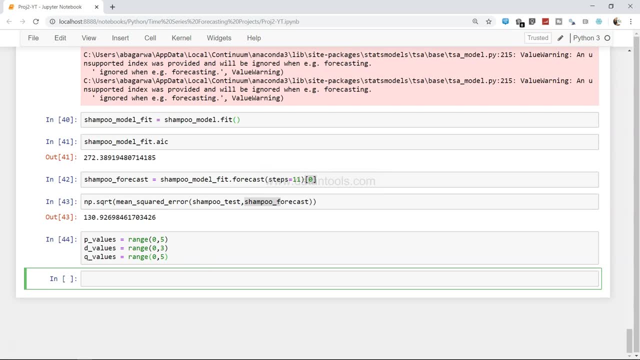 want to experiment between 0 to 5. okay, let's go ahead and execute it. and before I go ahead and execute this, what I need is basically, I want to import the warning, because it will. this process will show a lot of warnings. so import warnings and warnings, start. filter warning say ignore. this is a method if 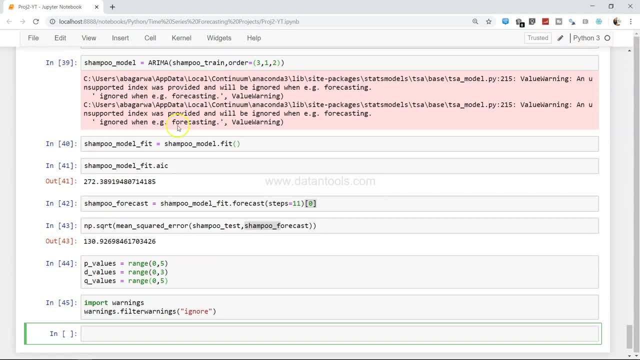 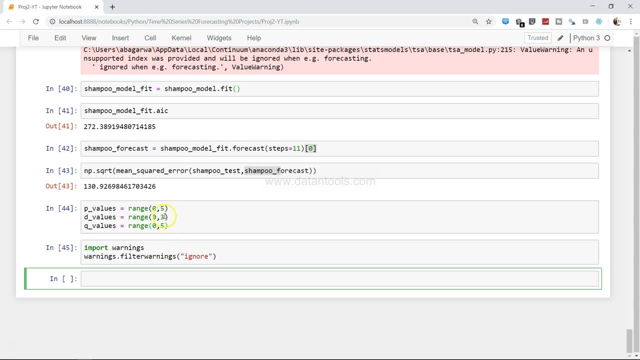 you want to ignore the warnings which I coming, like this one? okay, all right. so what I need is basically a loop where I can loop through these values. so, for P in P values: this I have already done in one of my previous video. I'm just doing it again and I have explained it in a 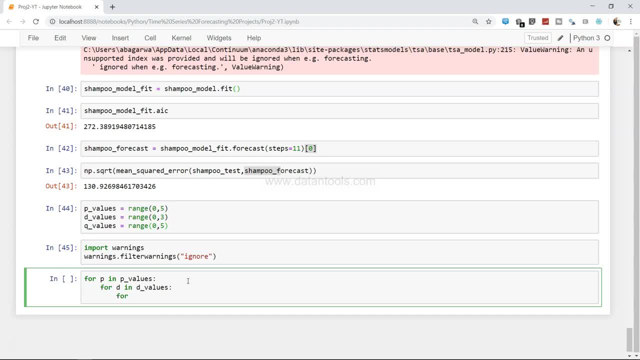 long detail that I am just iterating over PD and Q value in the same order in which they go into the, the order parameter of the Arima method. so P, T, Q. so this P is coming over here. so first the P is going so 0 and then this particular the iteration. 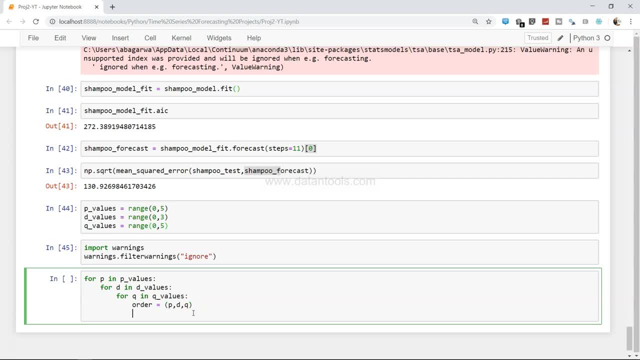 will happen and you will see the iteration also. so for now I'll just go ahead and say train and test and simply what I did earlier: shampoo zero to 25 and comma. shampoo 25 to 36, and then predictions equals to list. I want to store the prediction in a list so that I can test it in the using the test and I 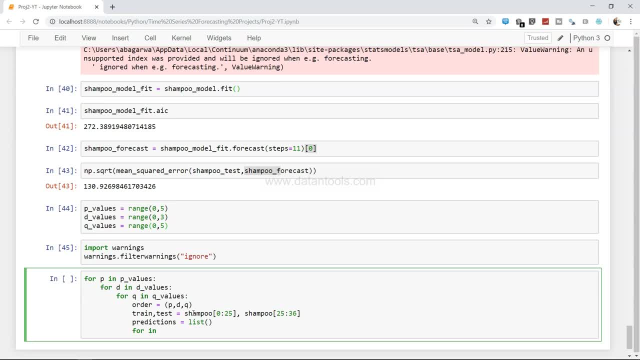 need to loop through number of times. the the test is basically there. so for I in I in range of alien test, right, because that's the number of times. we have the values into the prediction and we want to store it. so we need to loop it through by that number of times. so it is 0 to 11 that case and we want to in case, 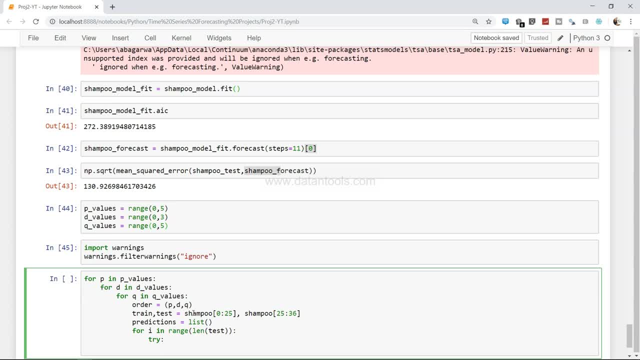 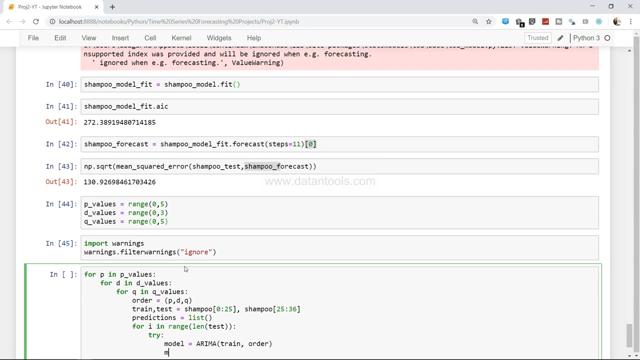 of an error. so you've seen that error has come earlier. we want to just continue when the error is coming and warnings will be removed in that case, because we have already filtered the warnings. Arima and train order model underscore: fit equals to model dot. fit, the ASP equals to 0. I have already explained in my 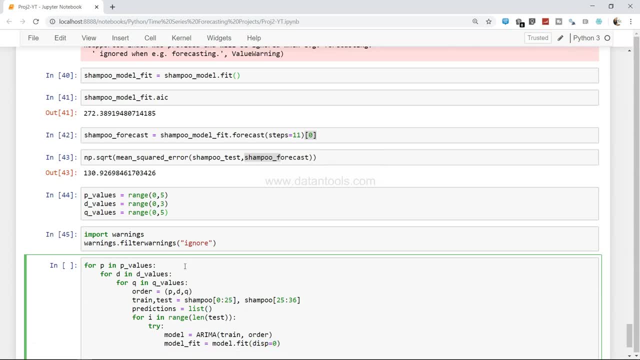 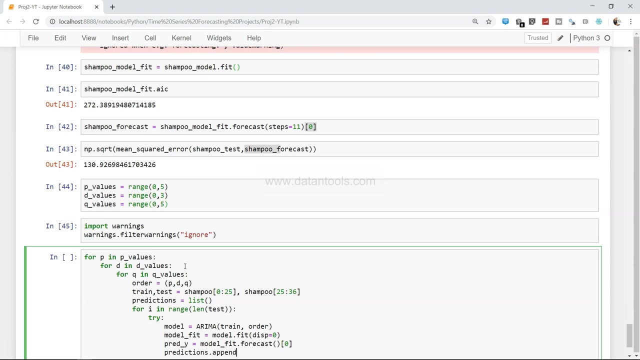 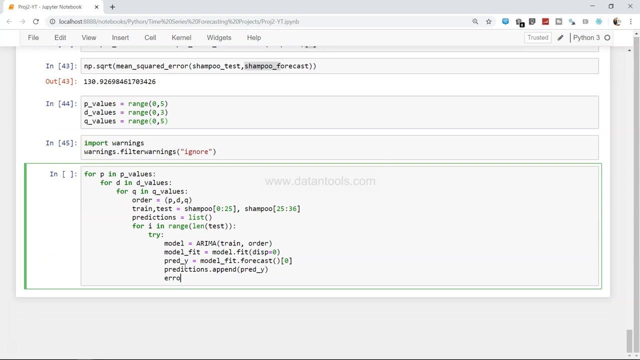 initial video about this particular displacement and then PR ed. underscore y equals to model dot. model the score fit dot. forecast want to get the forecast value which is stored in the first array, and then we say: predictions dot. append the predicted value, which we just did in the above statement, and then finally, what we have is the error which: 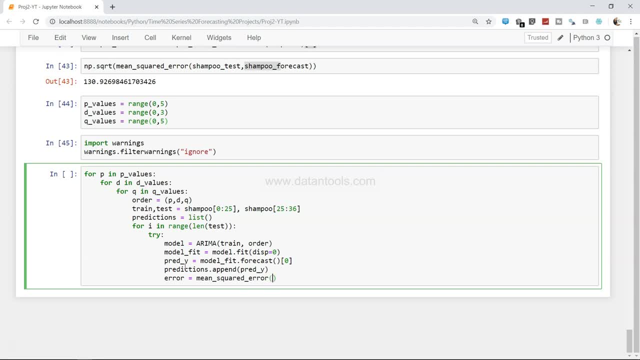 is mean squared error and say test predictions, and then we can print it: the re mom percentage s, because it is a streak, RMSE equals to up till to float value. we want right and it has gone: percentage. specify the order. this is our order dot. we have thought that we had order. well, what is? 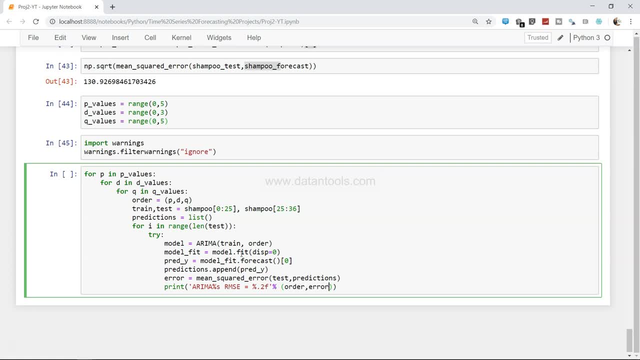 the order that we are calling right now. and what is the error? okay, you can even have colon, if you want, or if you don't want, that's also okay. then finally, for try, we say accept, continue. so we have just completed this model. i hope it should. 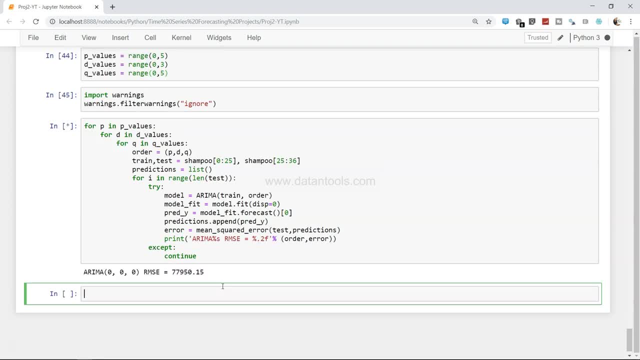 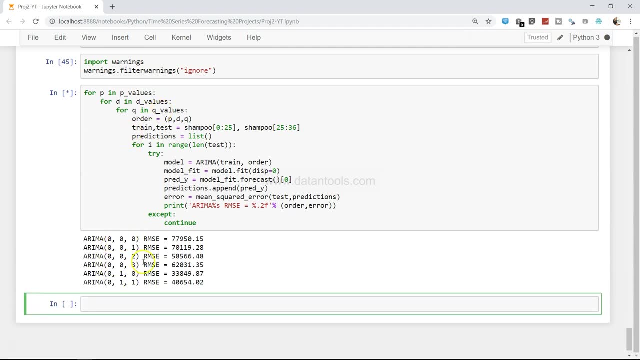 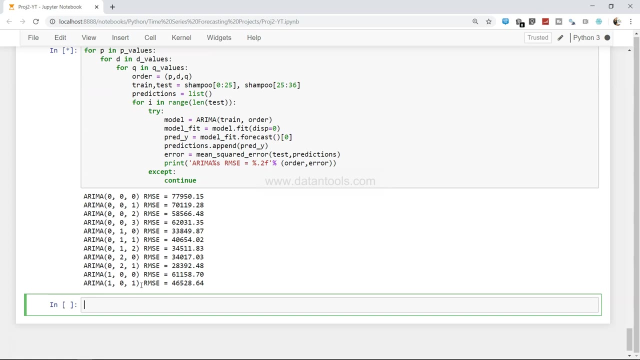 work fine and if i execute it, yes, so without any issue, it is, if you can see, zero, zero, zero, zero, zero one, which is q, zero, zero, two, zero, zero, three, right, and then zero one, zero, zero, one, one, and all of that. it's basically going on and showing you the different errors. so what we 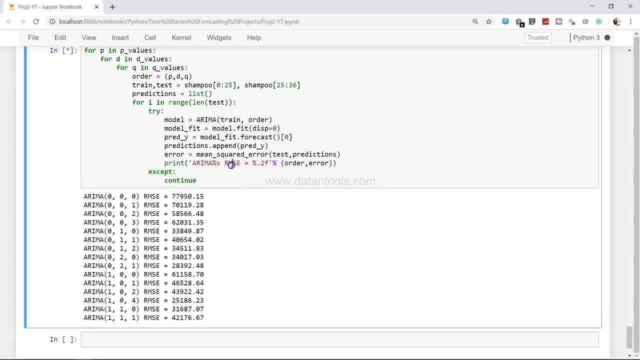 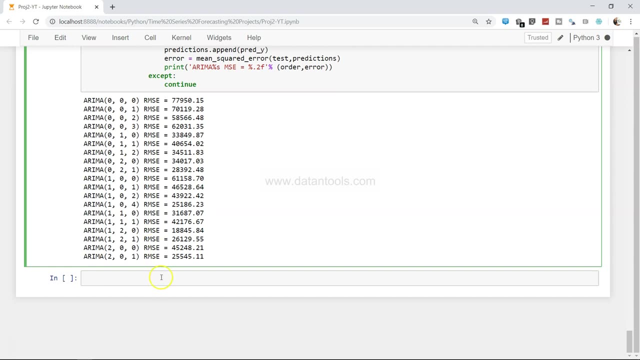 can take is not. this is not the rms root, this is just the msc. sorry, just the msc. so next time, whenever you run, say msc, not rmsc. i may be experimenting with earlier, so so rmsc is uh is something which we will try. so right now, the most smallest value we have got is 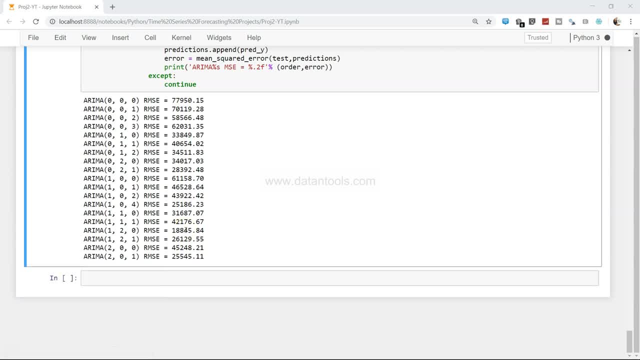 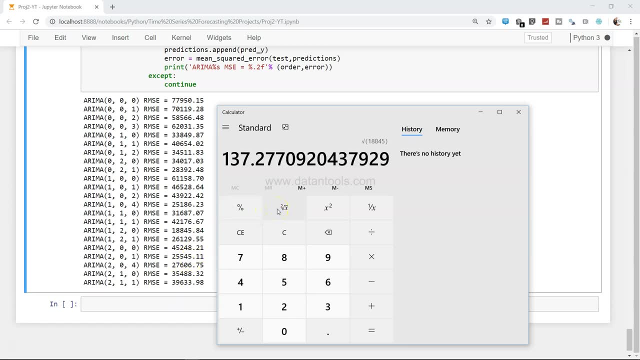 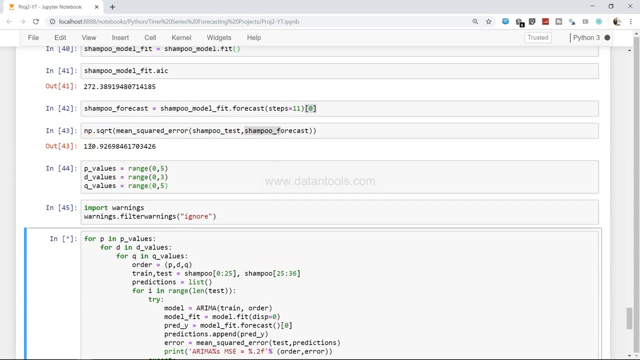 one double eight, eight, four, five. and if i just say calc one double, eight, four, five, and i take a square root of that, we get 137, and 137 is even higher than 130, which is even higher than our naive model. so our naive model is still winning, right. 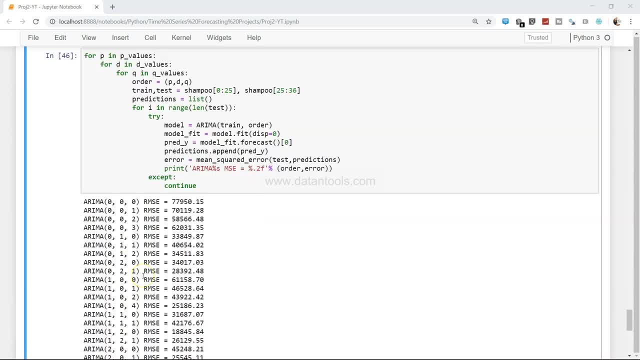 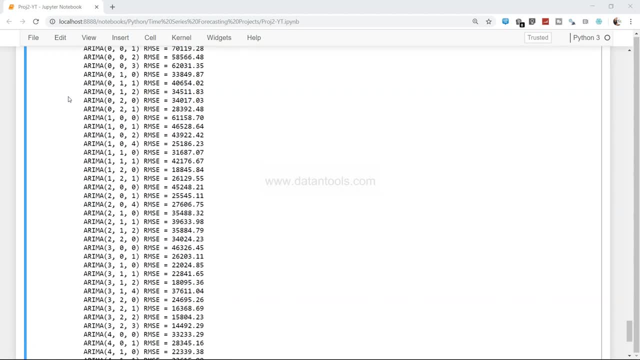 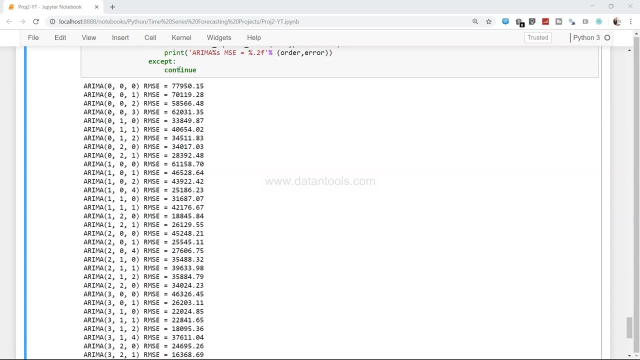 and it will take a minute, so i'll just pause the video. all right, so it has been completed. it took some time, but uh, like, for example, around two, two and a half minute to complete all the iteration. and if you see, if i just scan it through, though, there is a process that you can just have the 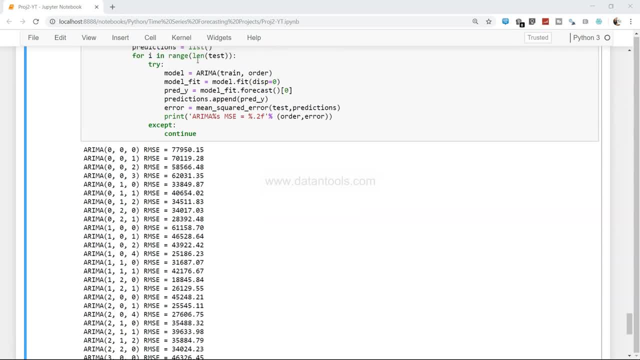 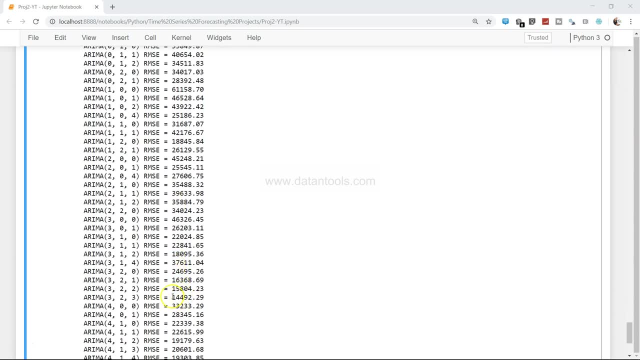 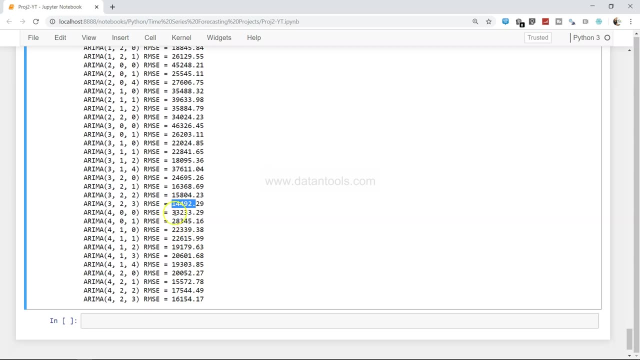 minimum. um, uh, you know the min parameter to get the minimum value of the error. but for now what i have is i can quickly scan through the error and i can just scan it through the error and i can just scan it through, as i was watching it. one, four, four, nine, two- is there anything smaller than this? 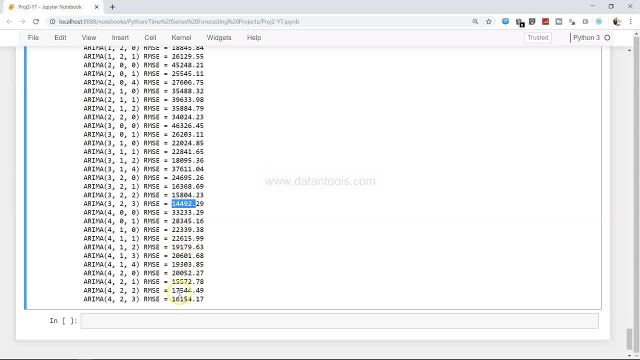 um, no, so this model- three, two, three- is our best model. so let's see whether this is smaller than the naive or not. one, four, four, nine, two, take a square, one twenty and one, 120 is the error that we get in case of Arima 323.. 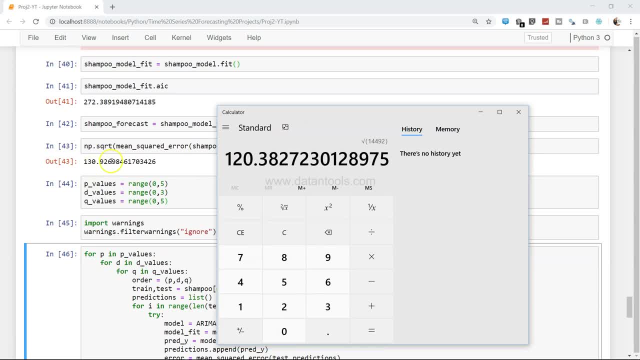 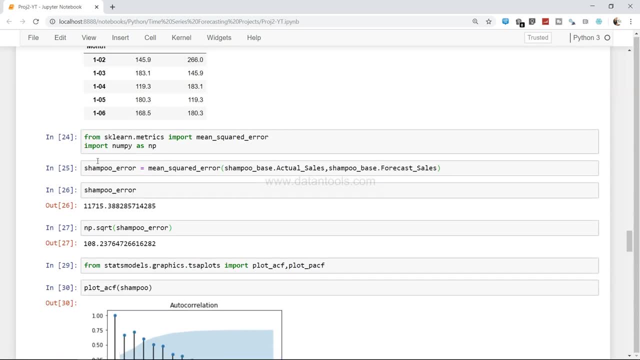 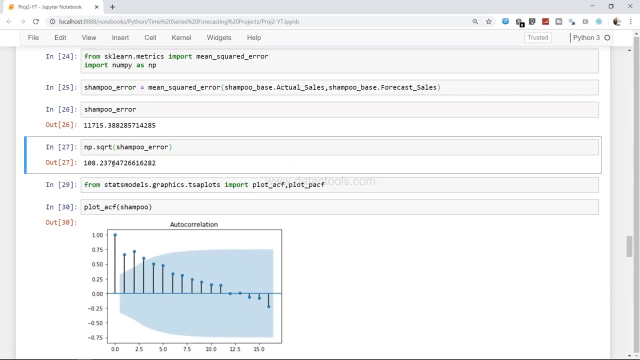 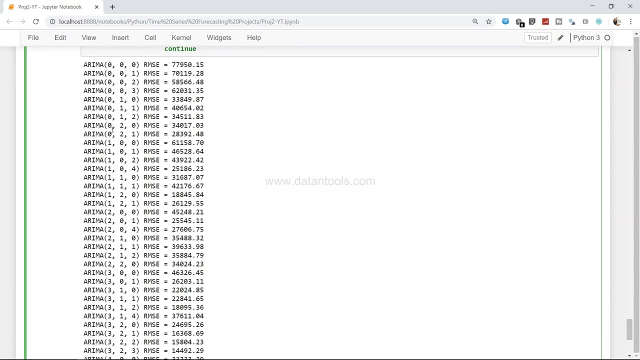 So 120, if I say 120,, over here it is 130.. So it's better, Right, Our previous Arima method. And if I say the naive, where is our naive 108.. So this model, even this model, which we have tuned it through the parameter, it is 120. 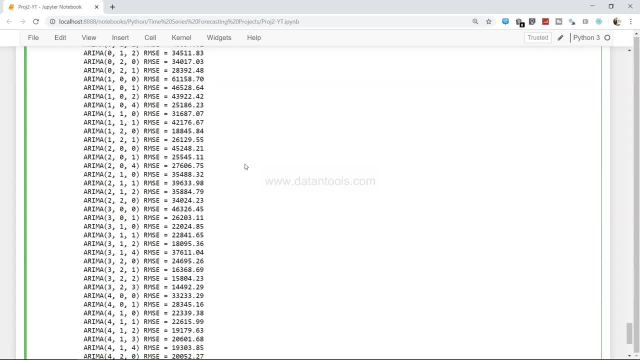 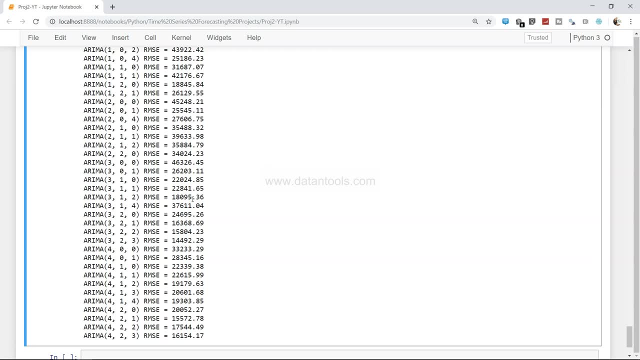 if you see, And still not better than the naive model. So we are going to reject it and we will just keep the naive model until and unless we find another, better model and that requires, let's say, the log transformation or another types of transformations that one can apply and figure it out, the right value.